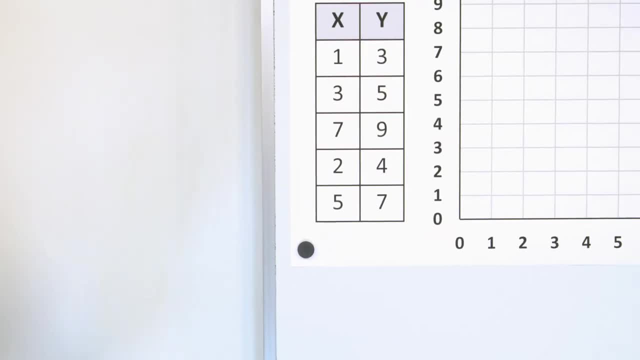 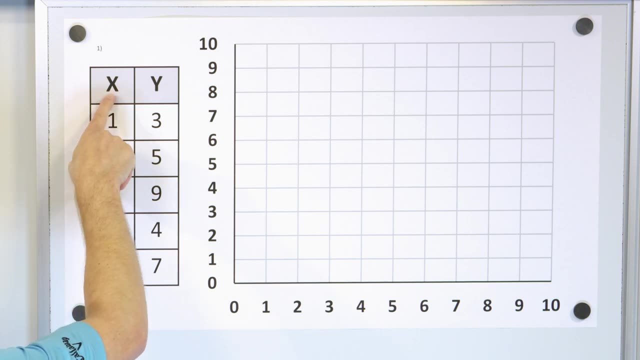 much time on graphing. That's the other thing we're going to learn here. So for our first problem, I think it's just going to be easier to jump right into our first problem. So here we have a bunch of points. You see, we have an x, we have a table here, We have an x column with numbers and we 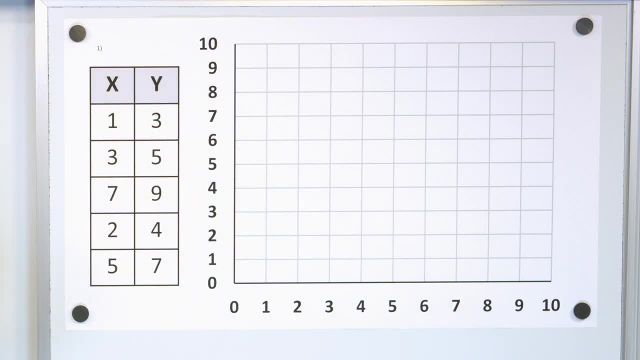 have a y column that also has numbers. Now, the way you need to read this, aside from the points, is that over here we have what we call an x- y plane, or, you might also see, called a coordinate plane. The thing I want to call to your attention here is that we have 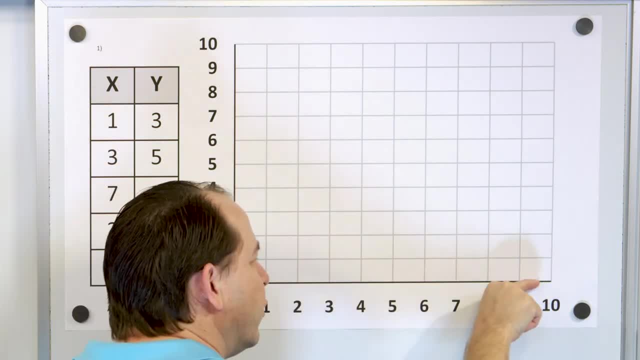 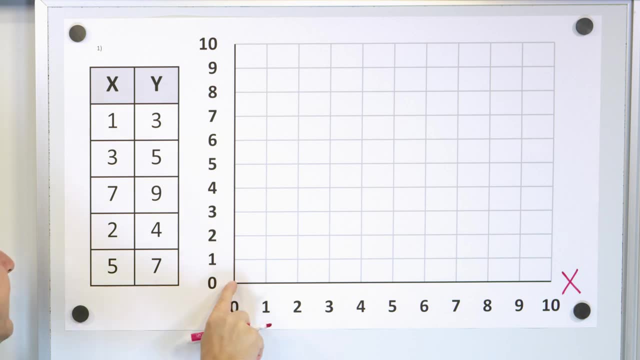 numbers in this direction, along what we call this line or this axis. The horizontal axis is what we always call the x axis, so I'll put x right there, And then the y axis or the vertical axis here, this vertical line, here we call it the y axis, so I'll put like a y right there. So if you see, 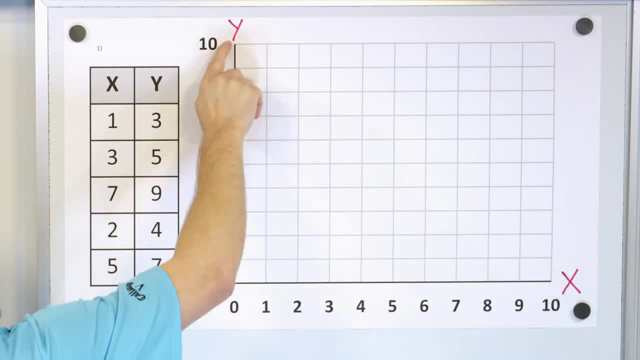 somebody telling you this is the x axis or this is the y axis, you automatically know the x axis is the horizontal, like this, and the y axis is always vertical. Now, if you only had the x axis, you would just be plotting numbers right here along this line. If you only had the y axis. 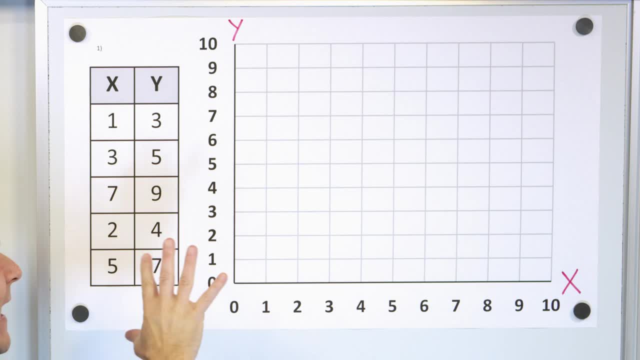 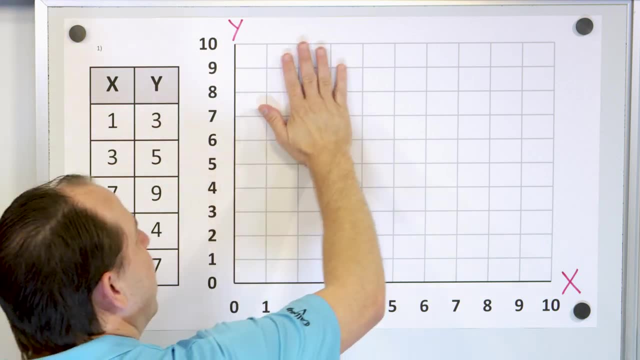 you would only be plotting numbers along the y line like this, But we have x and y together. So because we have x going this way and y going this way, when we put them together we have what we call an x- y plane. A plane is a flat thing, a flat surface. So when you see something called a, 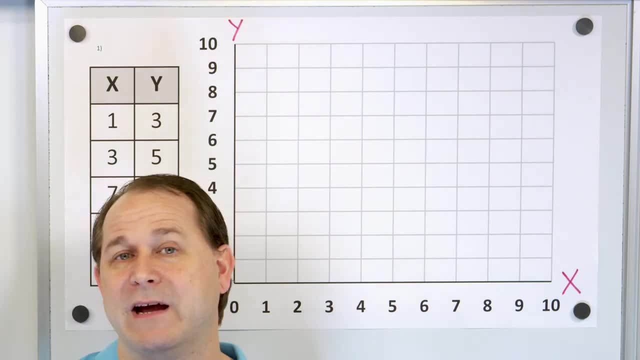 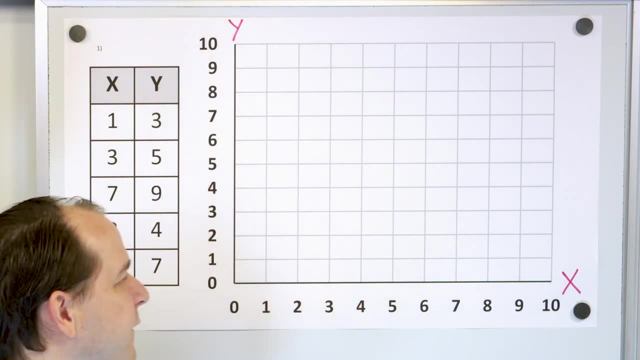 coordinate plane or an x? y plane, you can see that it's a flat surface. So when you see something called an x? y plane, or sometimes you see it called a Cartesian plane, that's another story why it's called that. It goes into the history of who invented it. Then all of those things are 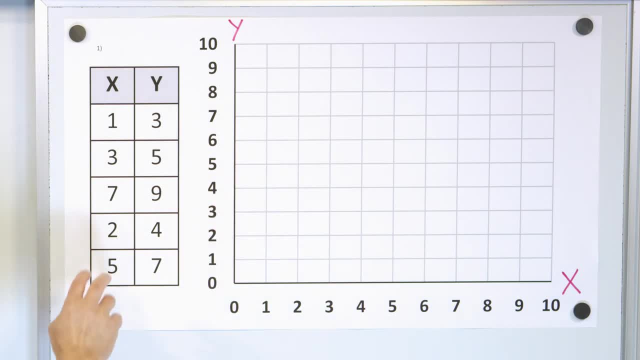 referring to the same thing. Now, here, what we want to do is take these numbers and represent them on here, plot them on there and understand what they mean. Here we have an x column and a y column. Now the way you read it is: these numbers go together as a pair, the x- y pair. These numbers 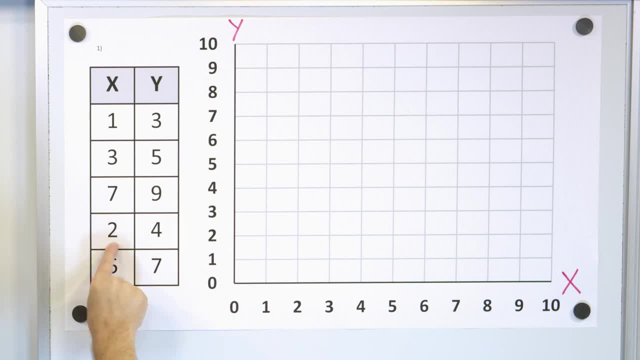 go together as a pair. These numbers go together as a pair, as a pair. as a pair, The x and the y, they're joined together as a pair. They're like partners. You can't really separate the x and the y values when we plot them. The whole point of it is that they go together in. 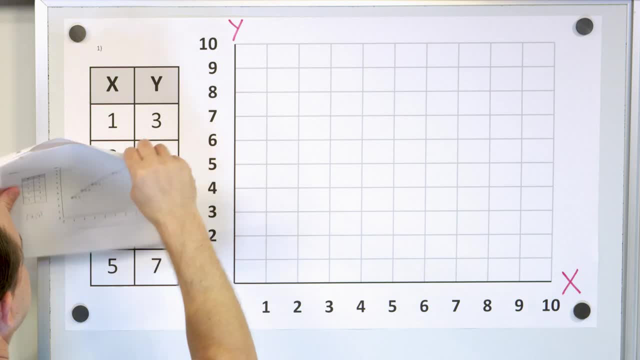 pairs. all right. So we look and cover up the rest of this table. The rest of this table means nothing. We're only going to look at this pair We have: x is equal to 1 and y is equal to 3.. So in 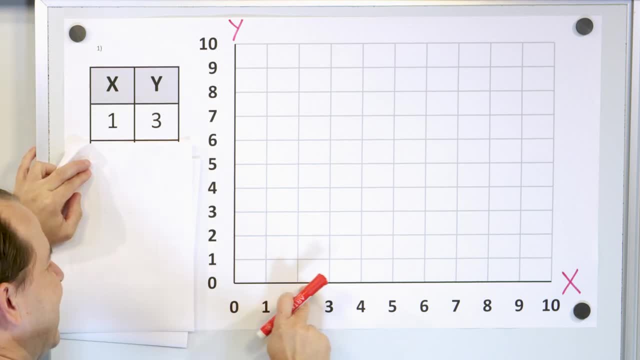 order to represent that point on the plane, we go in the x direction down here, only one unit over. That means we stop right here, because this is x is equal to 1.. So x is equal to 1 is right there. 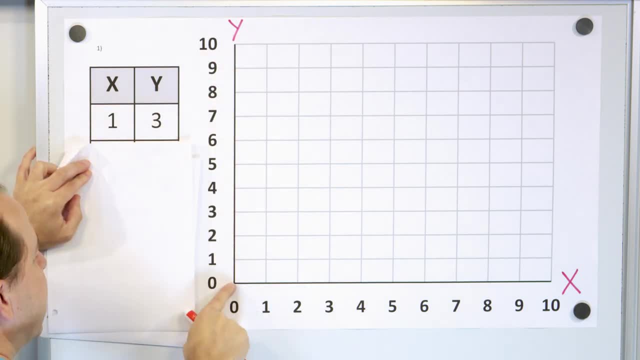 But y is equal to 3.. Notice, this is the y direction. So we go over 1,, which is this number, and then we go up 1,, 2,, 3.. You see it's right here And the intersection of these points. 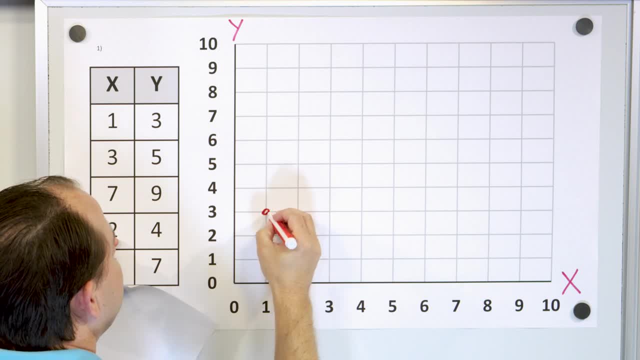 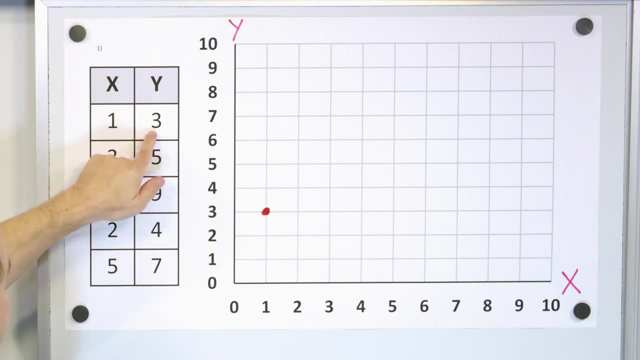 those lines there. that's where we put a dot 1, 3.. So we'll put a big fat dot right there. So what we have represented is that this point 1, 3, when x is equal to 1 and y is 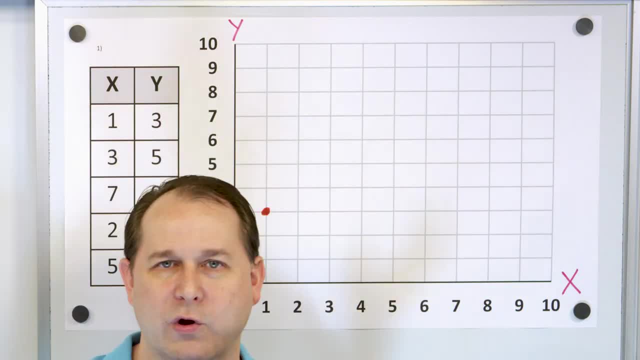 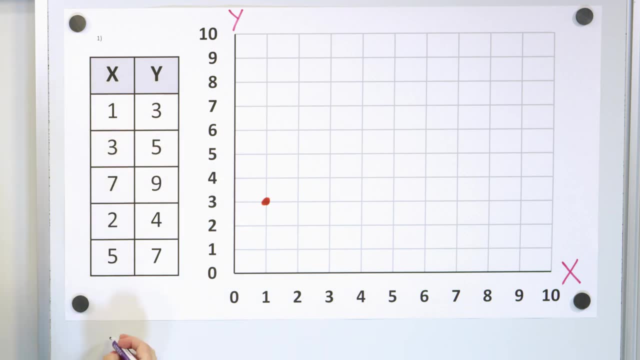 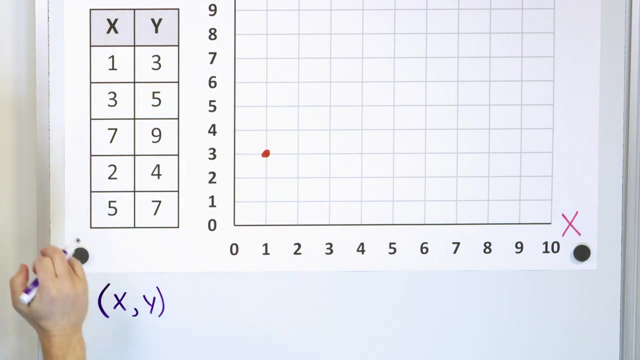 equal to 3 is represented by this dot on the coordinate plane. Now I'm going to take a second to jump down here and tell you that these- I have this in a table here- but what we often see in math is the points represented as a pair in parentheses: x, y. It's the same thing as this. 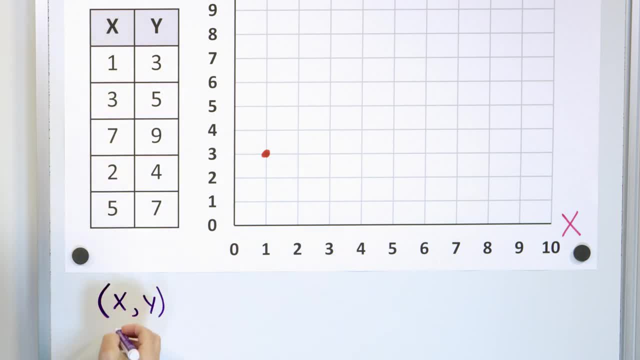 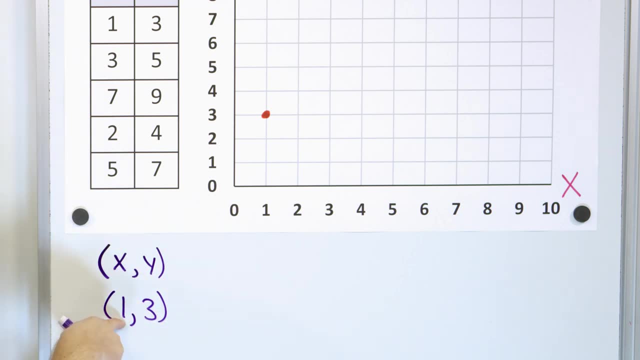 table. This first point in the table 1 and 3 would be represented as 1, 3.. So if you ever see a point- 1, 3, you know that the first number is always x, And the first number is always x And the second. 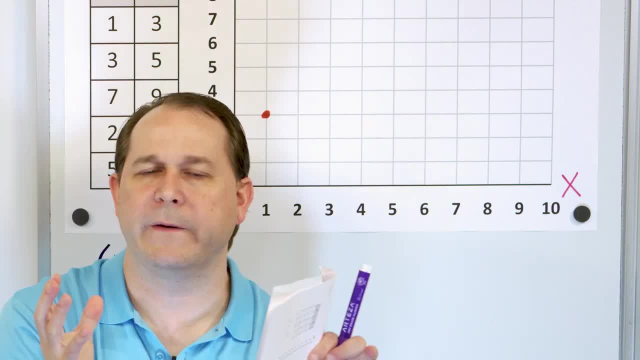 number is always x, And the second number is always x, And the second number is always x And the is always y. So when you see pairs of numbers in parentheses, the first number is x, the second number is y. So you go to: x is equal to 1, and remember, x is. 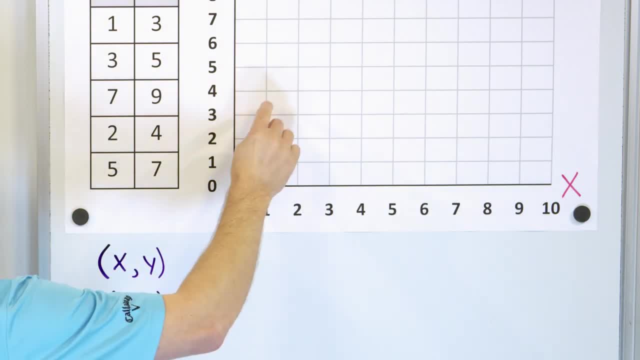 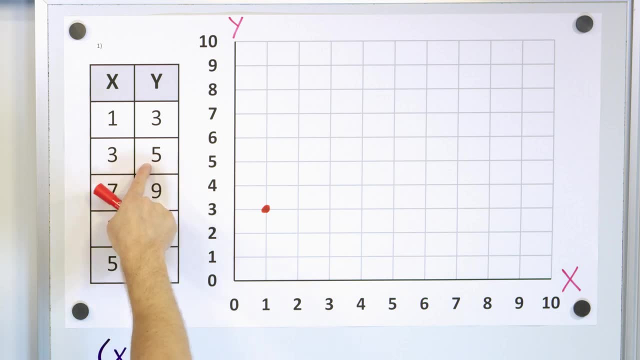 this direction and y is equal to 3.. 1,, 2,, 3.. And that place is where you put the dot. Alright? next point: We're going to ignore everything above and below. We're only going to look at 3,, 5.. So we know that x is equal to 3.. So we look in the 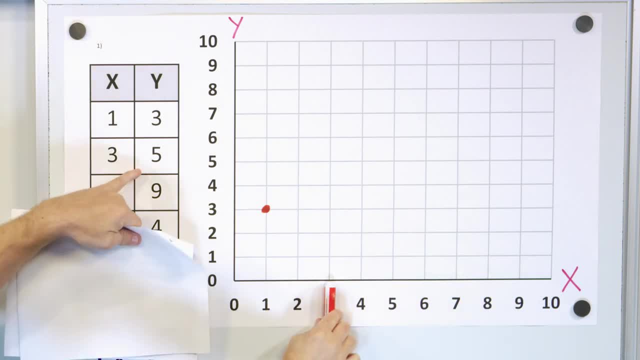 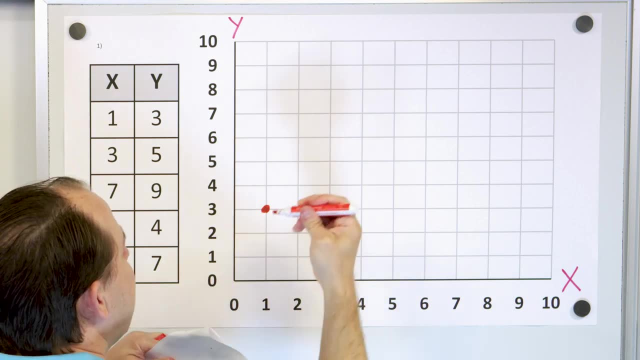 x direction 1,, 2,, 3.. That's x is equal to 3. And y is equal to 5.. We go up 1,, 2,, 3,, 4, 5.. Notice, we went to y is equal to 5,, x is equal to 3. And we put a dot. 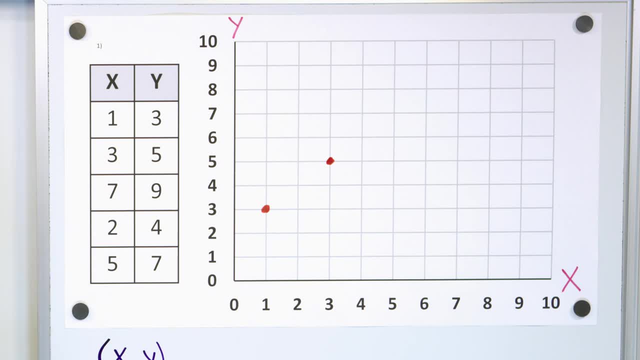 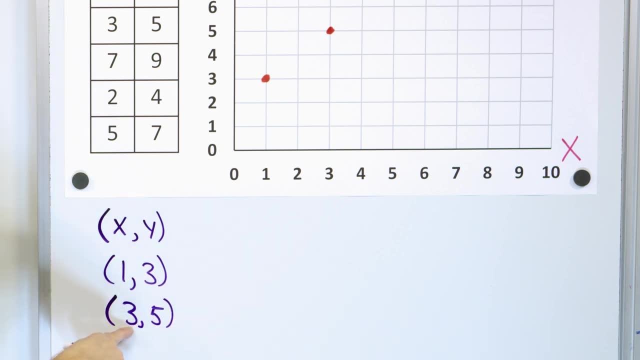 at this intersection point right here. If we were going to write this in parentheses, we would call it 3 comma 5.. And we already know x is equal to 3, and y is equal to 5.. That's how it's always written: x comma y. Alright, next We. 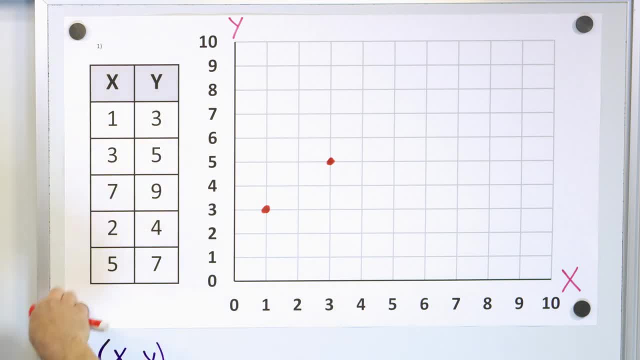 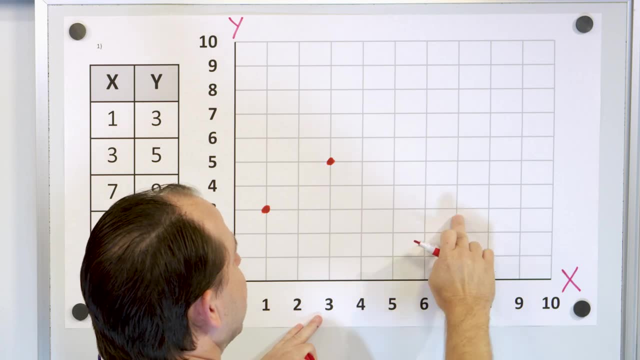 have 7 comma 9.. We know that x is equal to 7, and y is equal to 9.. So x is equal to you- just go to 7,, right, Right there- And y is equal to 9.. So we go up from here all the way up to 9.. Notice. 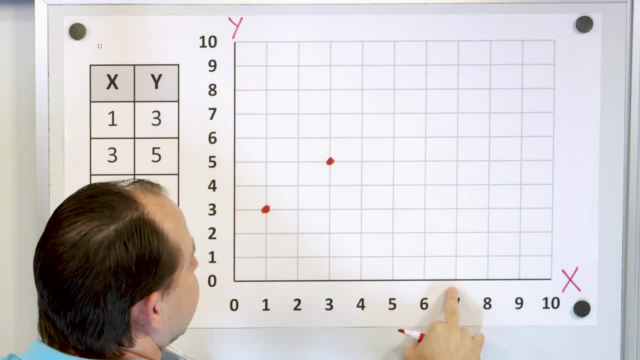 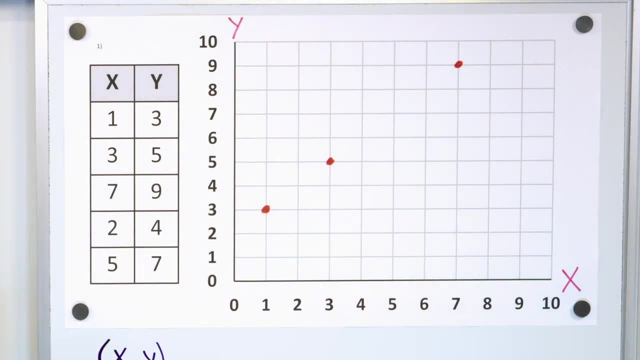 that y is equal to 9.. It's the intersection of these places right here. So 7 comma 9 means that we put a dot at this point, right here, Alright. Next we have 2 comma 4.. So x is equal to 2.. That's always the first, And y is equal to 1,, 2,, 3,, 4.. Right there. 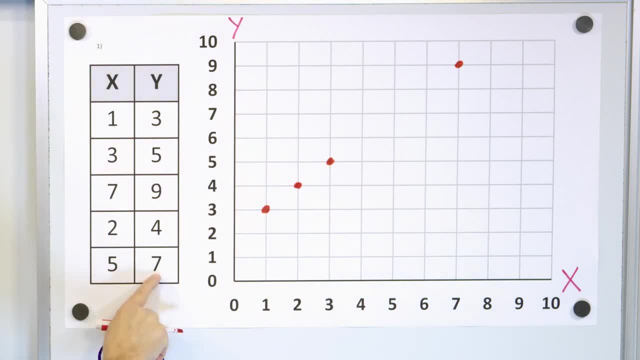 Which is a dot right there. And then our last point. Our last point is 5 comma, 7.. x is equal to 5.. 1,, 2,, 3,, 4,, 5.. And y is equal to 7.. 1,. 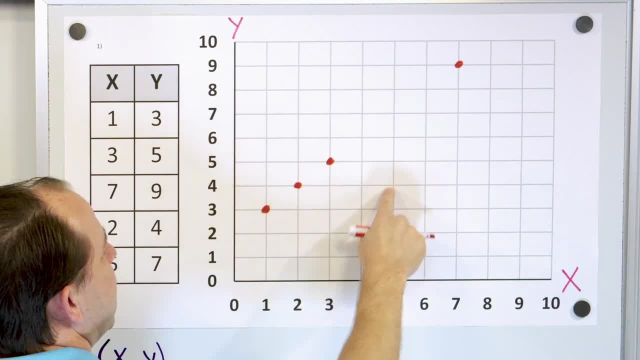 2, 3,, 4, 5, 6, 7.. Notice that that's the 7, and that's x is equal to 5.. So that final dot goes right here. So we have all the dots on the board. And if we wanted to write more, 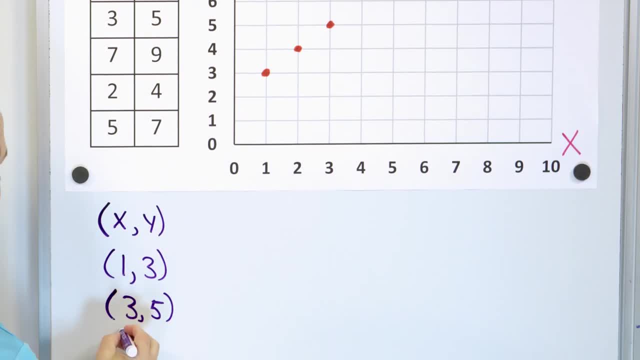 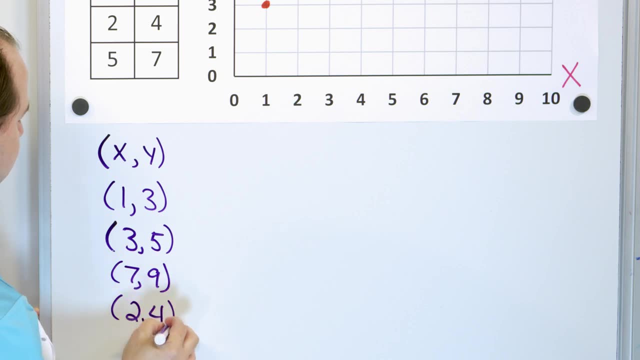 of these points, 7, x is equal to 7, and y is equal to 9 would be 7 comma 9.. And then x is equal to 2,, y is equal to 4 would be 2 comma 4.. And then x is equal to 7, and y. 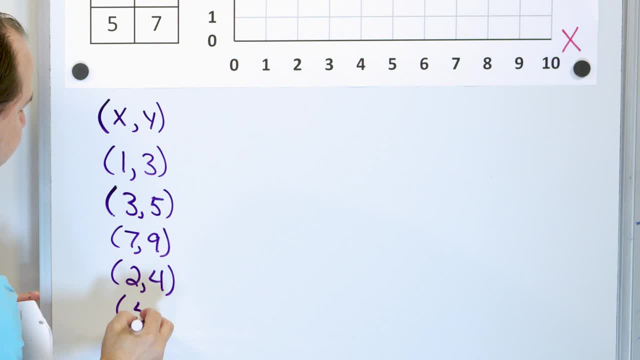 is equal to 4.. And then x is equal to 5, and y is equal to 7 would be 5 comma 7.. So you can put it in a table form or you can just write the points down. The first number's: 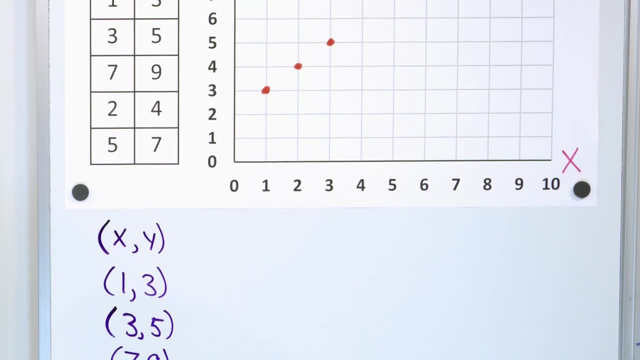 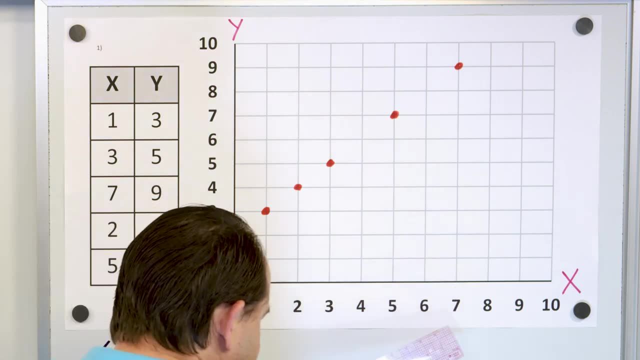 always x. The second number's always y. Now, in this case, what does this look like? This is a straight line of points. It's kind of nice really when you look at it. It's not going to be perfect. I'm not going to be able to draw a straight, perfect line, but I want. 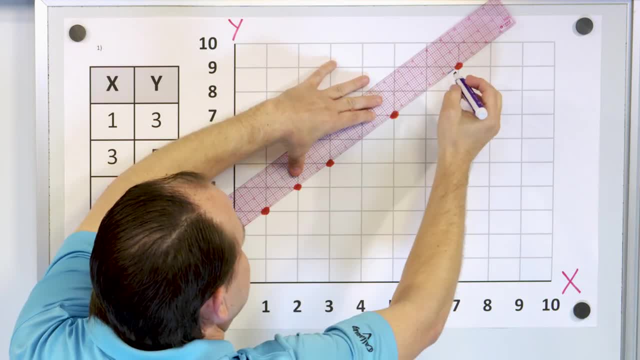 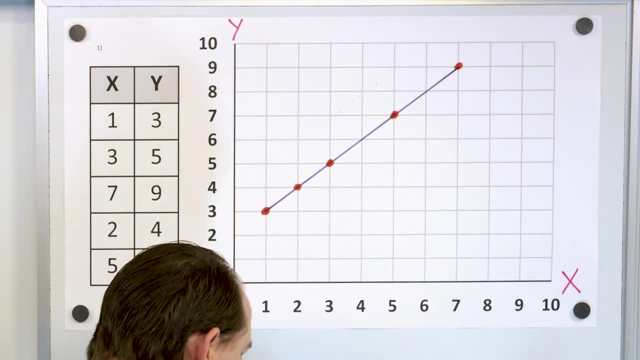 to try to at least draw and connect these dots. So it's kind of like back when you were and you used to play connect the dots. You get to draw lines and connect the dots. All right, so that is our line And you can as we go through math. 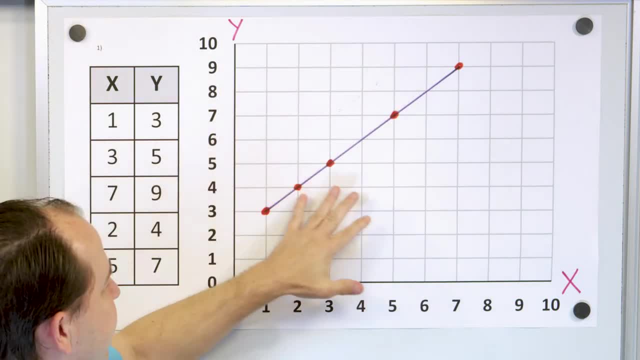 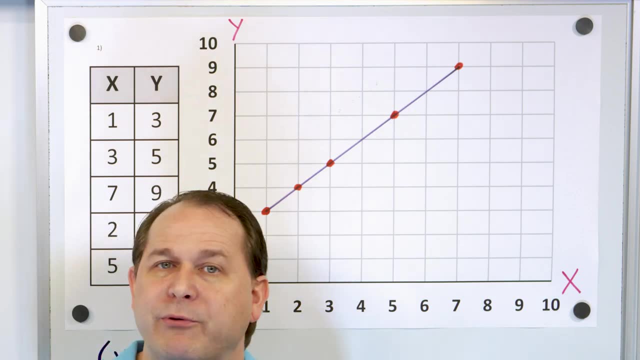 you will find that you can make all kinds of shapes on these planes like this. We are always very interested in lines because in real life lines represent lots of things in real life, but we also have other shapes that we'll learn about later. 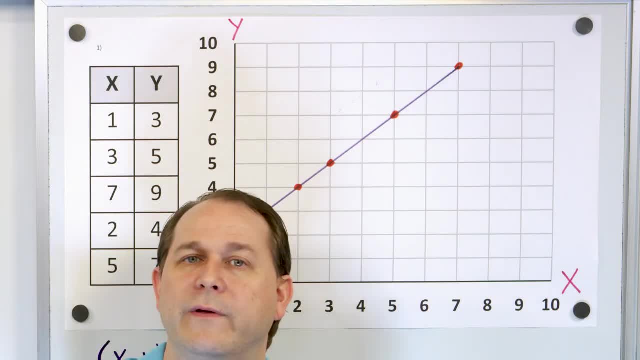 You'll see, even in this lesson here, we'll have other shapes that happen when we connect the dots. Now I wanna spend a minute to talk about what this could actually mean. Why do we connect the dots? Why do we need to do this? 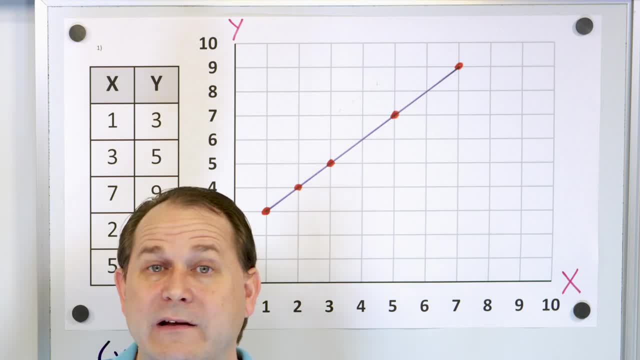 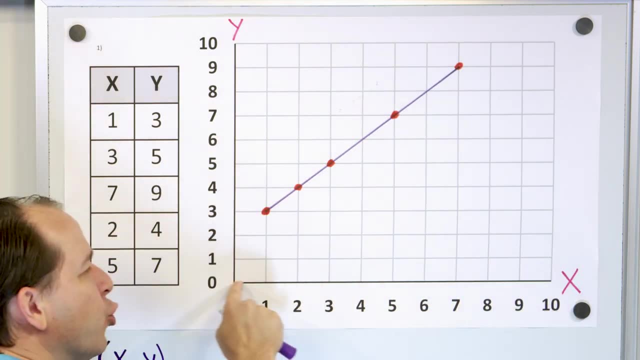 Why are we plotting things? So I wanna anchor it in your mind with a real example. Let's say we can make up anything we want. So let's say that x here really represents time in seconds. So this is. let's say, I start a watch. 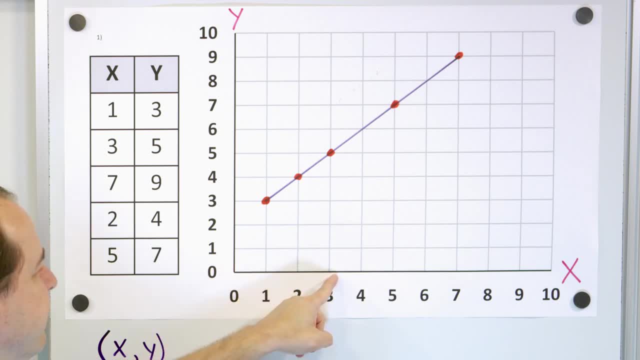 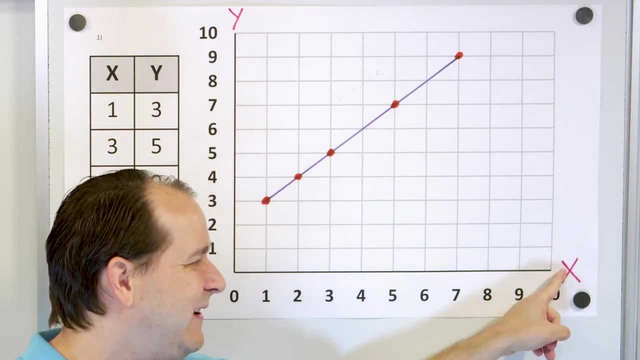 then this is one second, two seconds, three seconds, four seconds, five seconds, six, seven, seven. So time is represented down here on the x direction. You could call it t instead of x if you want, And let's just say for this example: 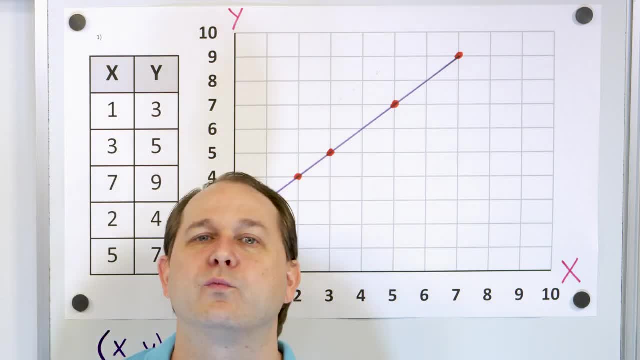 that y is representing the temperature in this room. okay, The temperature in this room. So I know the numbers are a little bit weird, but let's say that I start my watch. at one second after I start my watch, the temperature is three degrees. 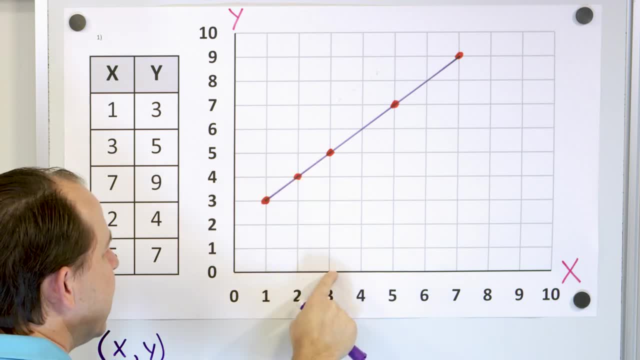 But then at two seconds the temperature is four degrees, And then at three seconds the temperature is five degrees, And then, when I skip down to five degrees, the temperature was seven degrees, And then, at seven seconds, the temperature was nine degrees. 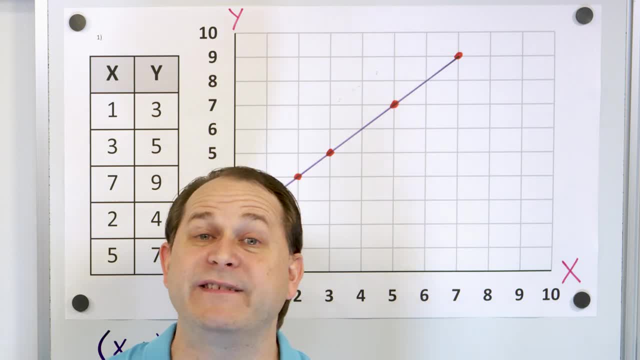 What does this graph represent, then? What it's representing is a room that is warming up. That's what it's representing. We start the clock. one second, two seconds, three seconds, four seconds. look, four seconds will be about here. 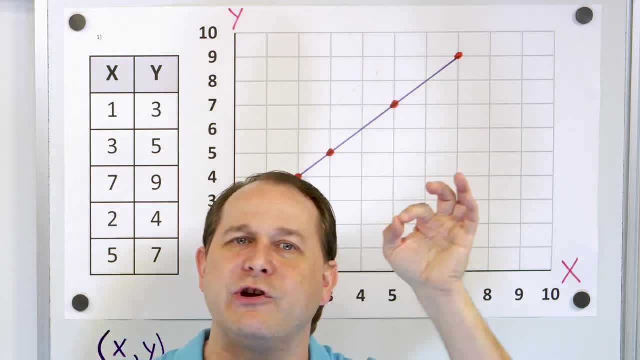 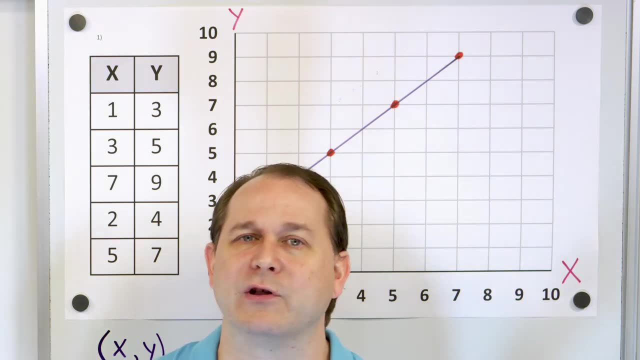 Five seconds is here and so on, And at every second we start a clock, the temperature is going up by the same amount. That is an example of what this graph could represent. We can represent graphs for lots of things, but the reason we actually use graphs 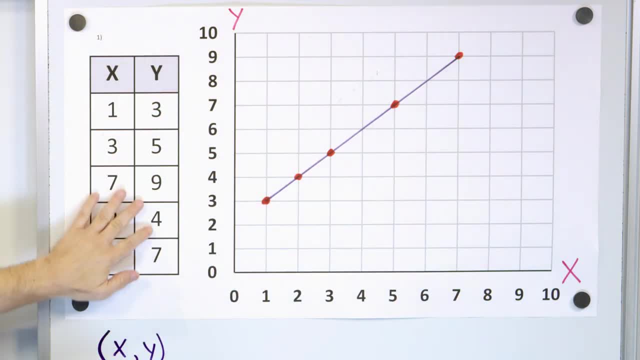 is because we can visually see. If we just look at the numbers, it's hard to see what's happening Like. can you tell me what's going on here? It's very hard to look at this and know what's happening. But when I look at a picture, 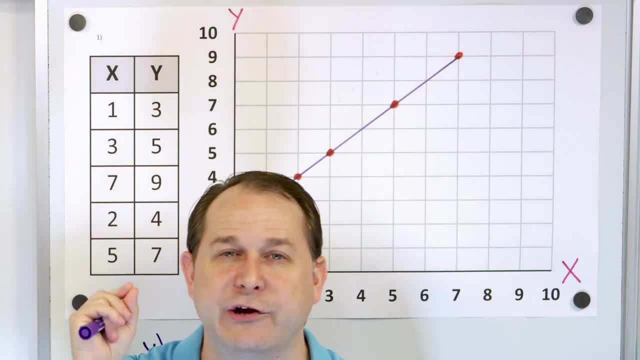 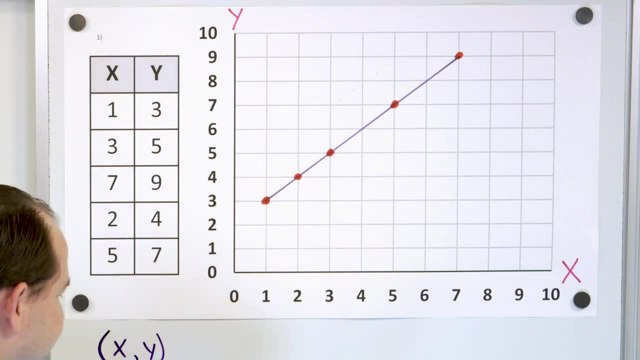 I know immediately: the temperature is increasing. And not only is it increasing, it's going up the same amount every single second. That's why we use graphs, so we can visualize things. All right, And one more thing I'll say. if you want to, you don't have to. 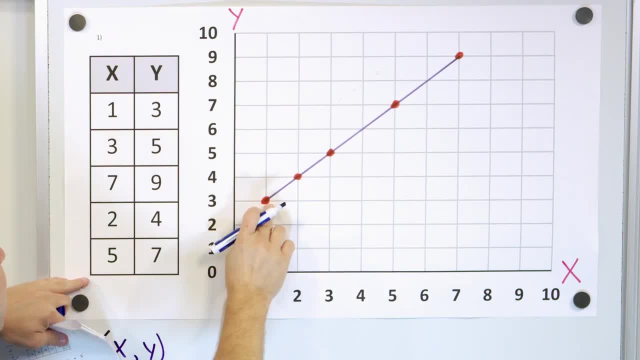 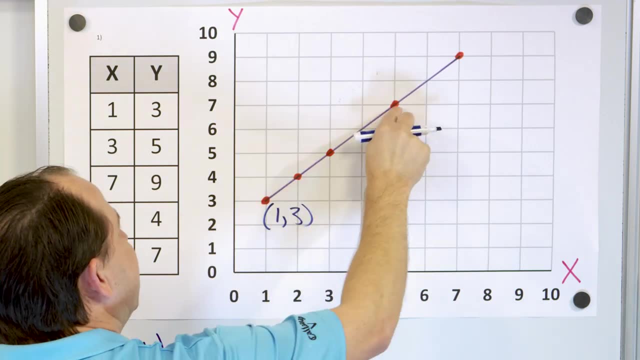 you can label the points on the graph. I mean, we didn't do it here, but this is 1 comma 3.. That was this point. So we could put a parentheses 1 comma 3 for this point here and we could label each one if we wanted to. 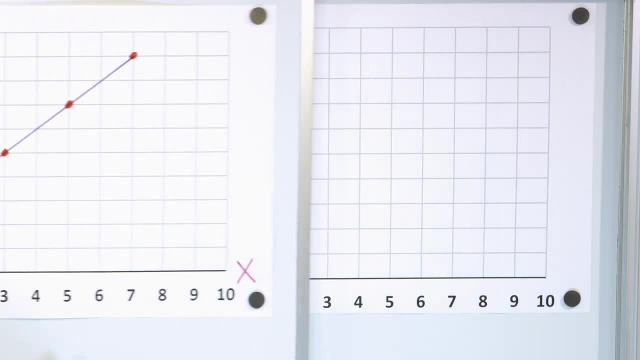 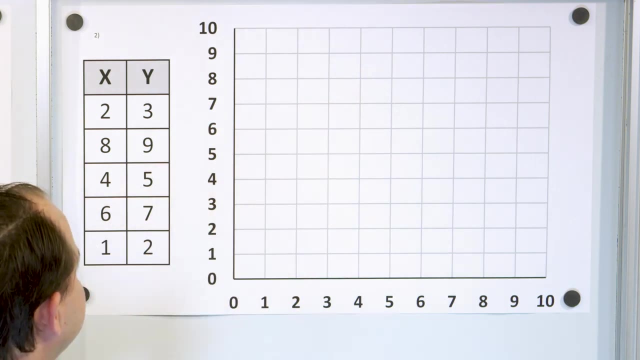 but you don't, of course, have to. All right, let's take a look at the next set of numbers here. Here we have another table and we have another blank, So let's go ahead and plot these points and see what kind of shape this one makes. 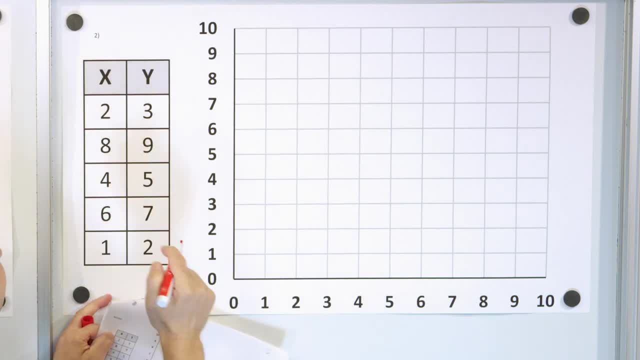 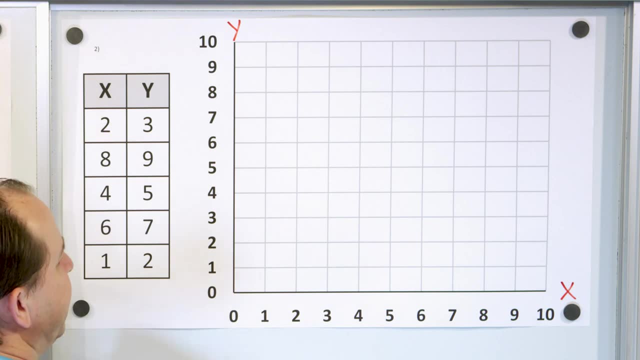 All right, 2 comma 3.. That means x is equal to 2,, y is equal to 3.. So x is equal to 2 goes this way. Remember: this is the x direction, And then up here is always the y direction. 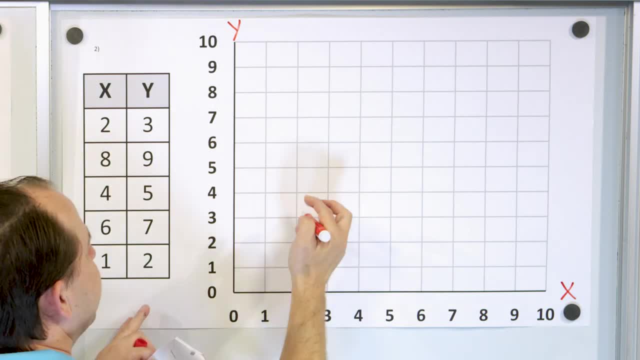 So x is equal to 2,, y is equal to 1,, 2, 3, which means there's got to be a dot right here. And don't forget, I'm not going to do this for every problem, but if you wanted to write this as a coordinate point, 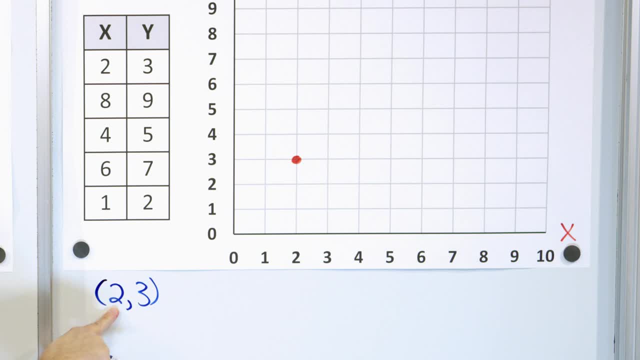 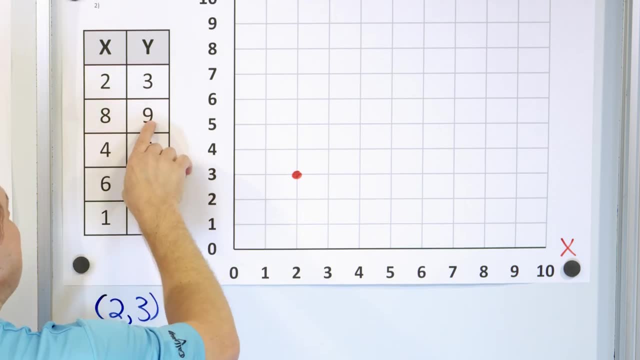 you would say 2 comma 3.. This always means the first number is x is equal to 2, and then the second number, y, is equal to 3.. All right, next point: 8 comma 9.. That means x is 8 and y is 9.. 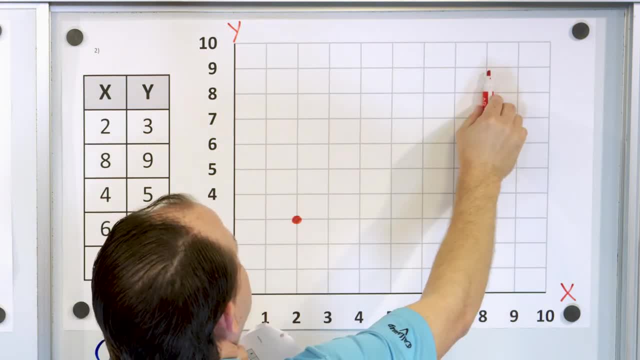 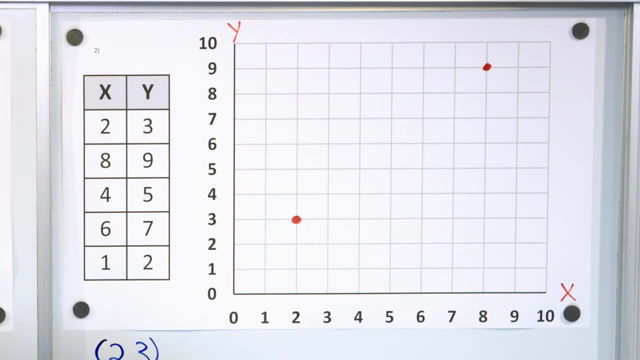 So let's go over to: x is equal to 8, and y is equal to. you can see right there: 9,, y is equal to 9,, x is equal to 8, and we put a dot right there. Next point, 4, comma 5.. 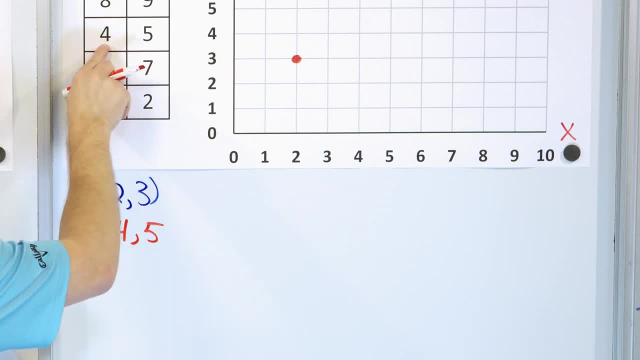 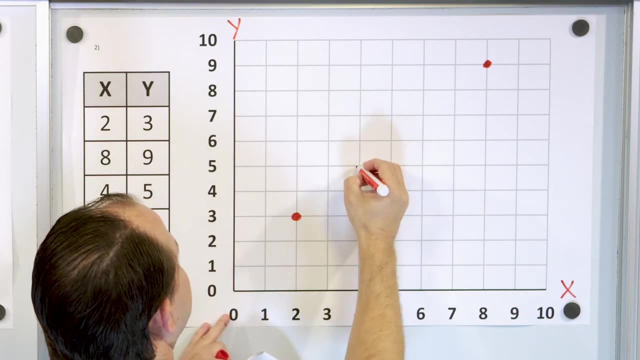 You could write that down as 4 comma 5.. That means x is 4, y is 5.. x is 4 is right here. y is 1,, 2,, 3,, 4, 5, which means a point would be right there. 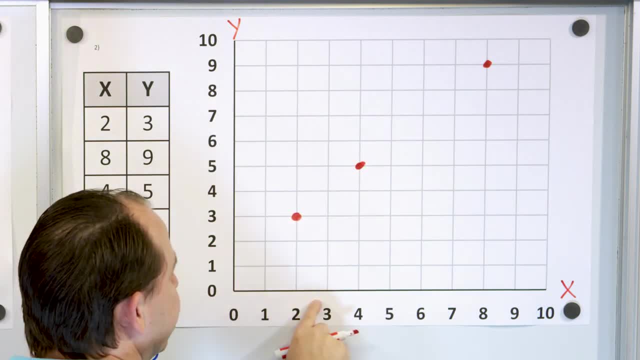 Next 6, comma 7.. x is equal to 6, 1,, 2,, 3,, 4,, 5,, 6, and y is equal to 7, 1,, 2,, 3,, 4,, 5,, 6,, 7.. 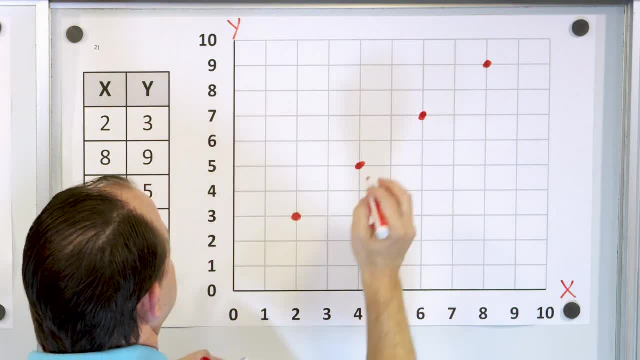 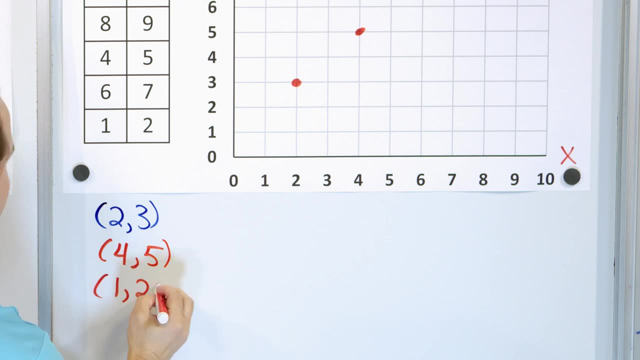 Notice that y is equal to 7 right there, when x is equal to 6.. Final point: 1 comma 2.. That means x is 1, you can write it like 1 comma 2, if you like. like this: 1 comma 2 is x is 1,. 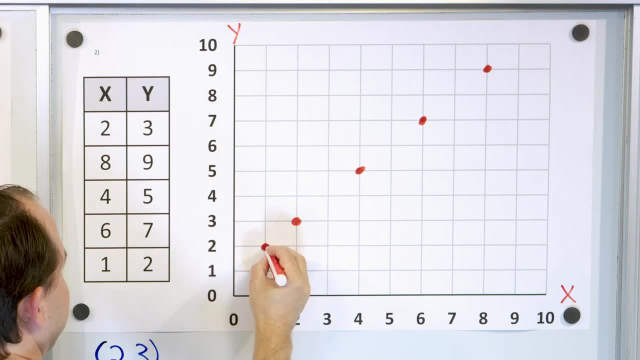 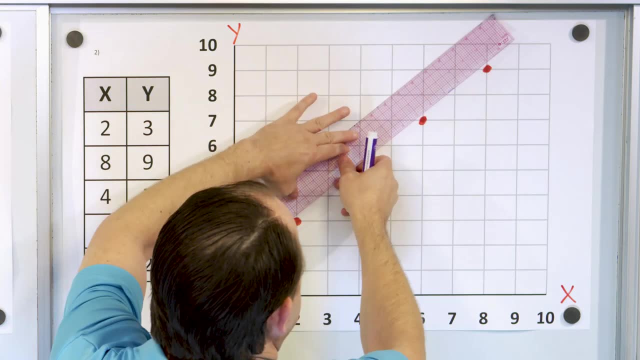 y is 2, and that means that this point is right here. So again, I won't do it for every single problem, but let's try to draw and see what this actually looks like. If I line it up, it's not going to be exact. 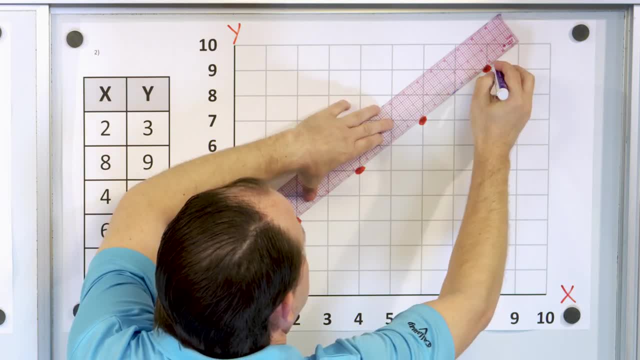 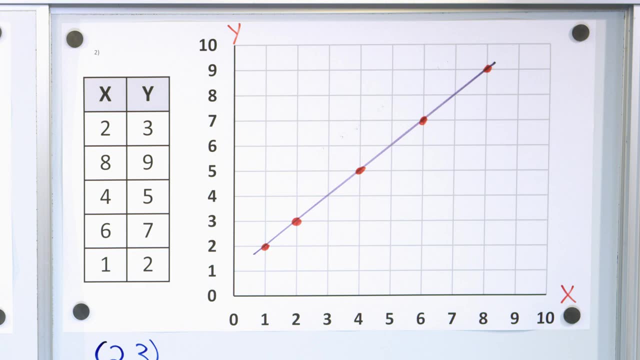 it's not going to be perfect, but that's okay. We don't care about exact, we just care about trying to understand what's happening. This is a straight line also that goes all through those points. So here again we have points plotted. 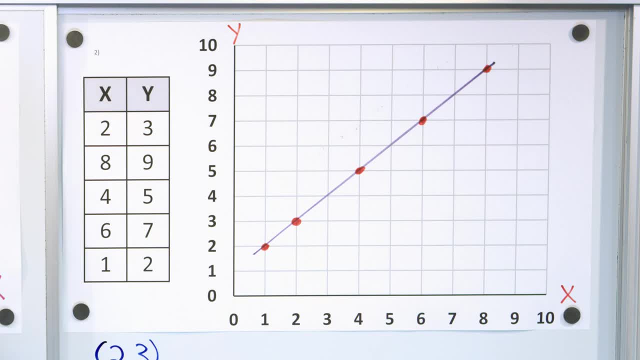 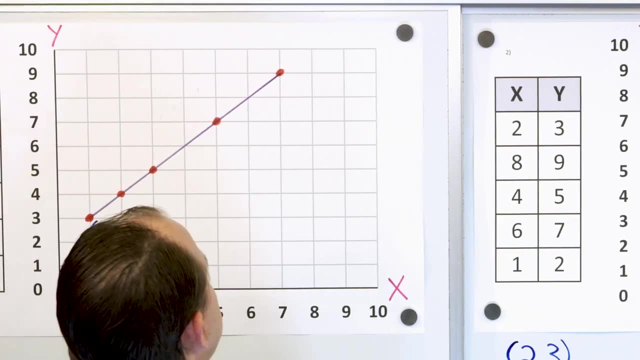 and they make a slanted line, just like in the first example. We can actually compare them and we can see the shape of that line looks more or less the same, but it's not exactly in the same location. This line is maybe shifted up a little bit. 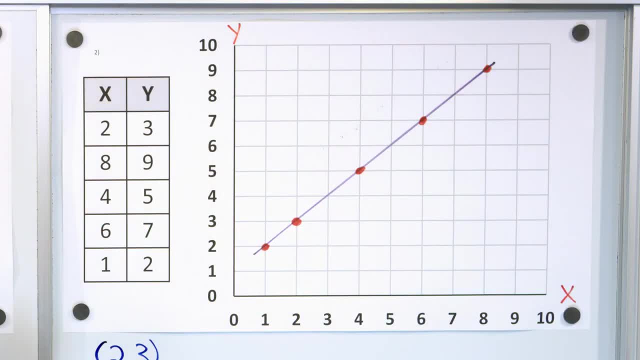 this line is in a different position, but the slant of the line- we call it the slope of the line- is basically the same. What could this represent? Of course, it could be temperature time here in temperature, but it could also represent something else. 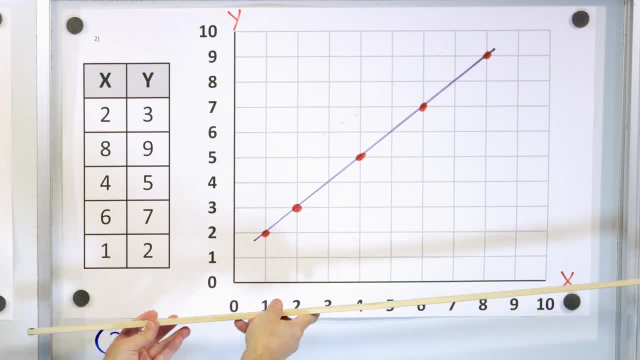 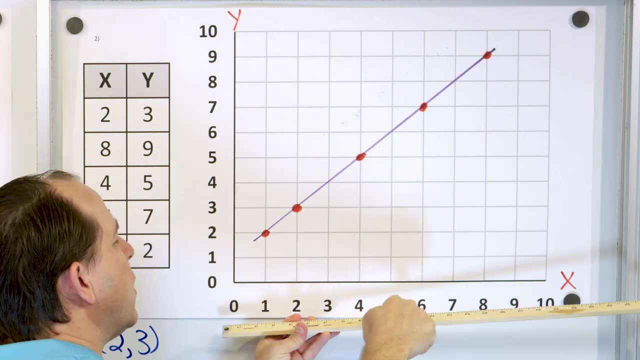 Let's say, just making this up, let's say I had a rod like this and this distance here, this, this, these numbers along x could be the distance along the rod. So literally this direction here is like a rod right here. 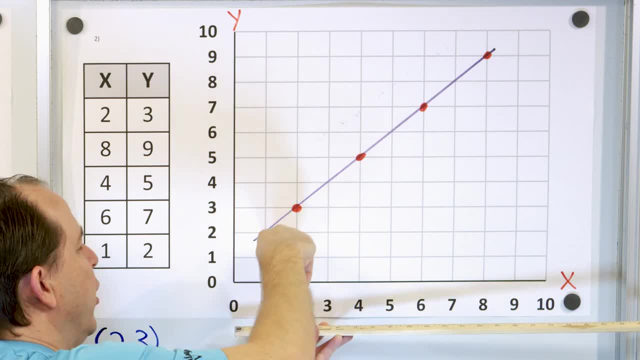 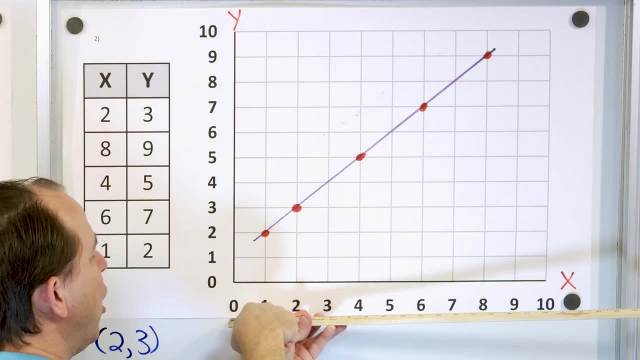 And then what am I plotting down here? I could be putting rocks on this rod, and the number here is telling me how many rocks I have at each position. So at one centimeter over, I might have two rocks piled here. At two centimeters over, 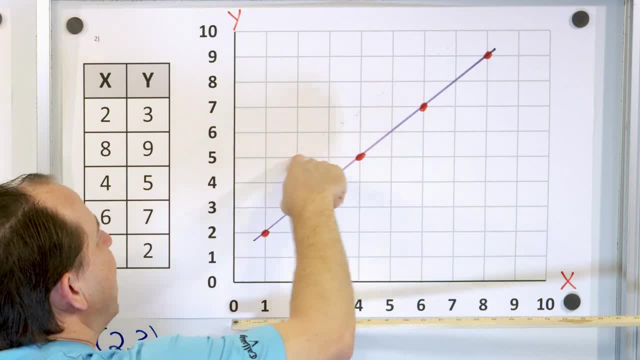 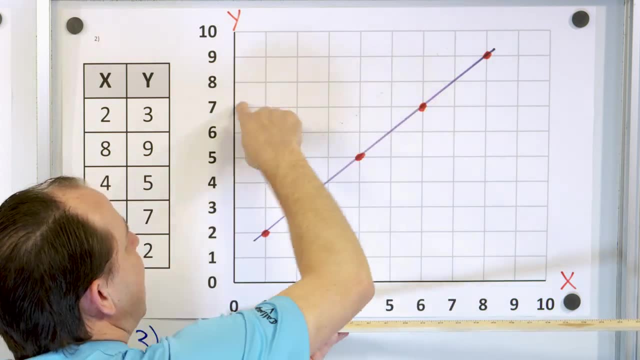 I might have three rocks piled. At four centimeters I might have five rocks piled. You see the pattern here. At seven centimeters down over here I might have. or six centimeters, I might have seven rocks piled. So what it allows you to do, 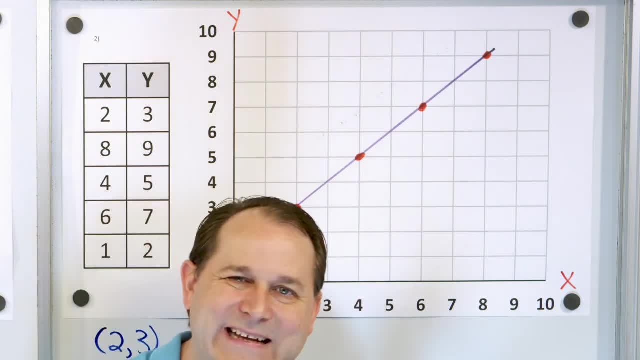 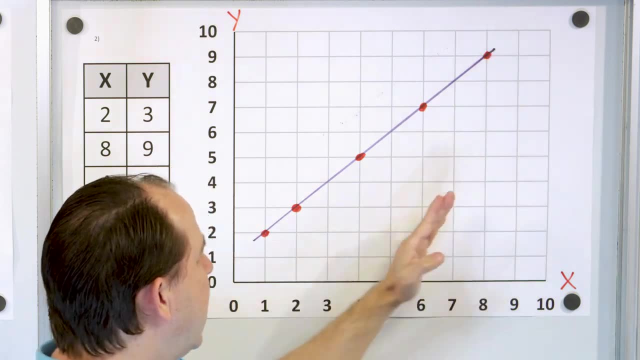 depending on what you're talking about is. I can look at a picture and I can see: oh, I have fewer rocks here at the end of the rod and more rocks over here near the other end of the rod, And the amount of rocks along the rod is going up, up, up, up up. 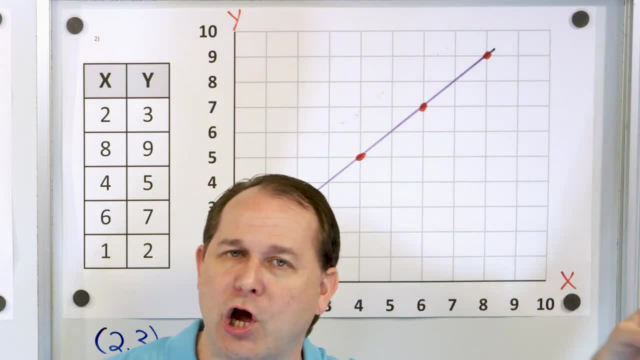 at the same number of rocks as I go along. In other words, it's going up at the same amount as I go down the rod. Alright, now let's change it up a little bit and do something different than a line. This one's going to be really interesting. 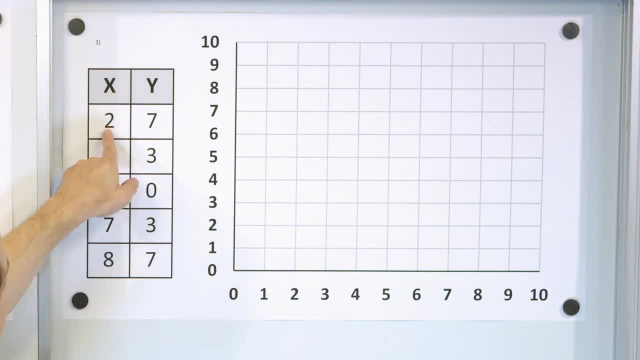 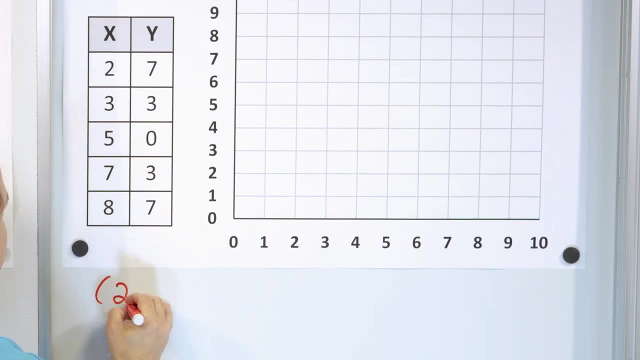 so pay attention to this one. Here we have points. of course, Two comma seven is our first point. So x is equal to two and y is equal to seven. If you wanted to write that as a point with a parenthesis, it'd be two comma seven. 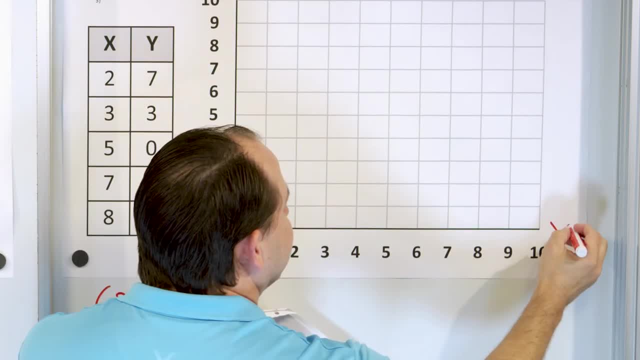 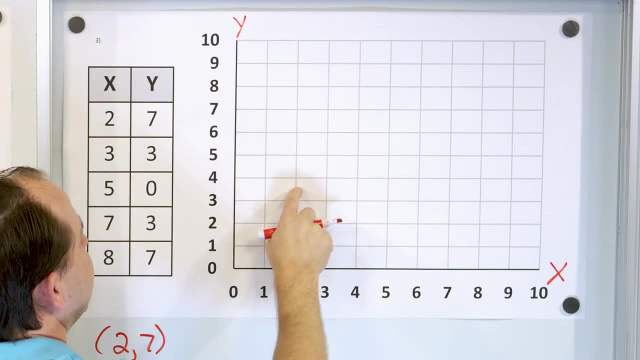 You write that as x is two, y is seven. So again, the x direction is here and the y direction is always up and down. x is equal to two, y is equal to one, two, three, four, five, six, seven. 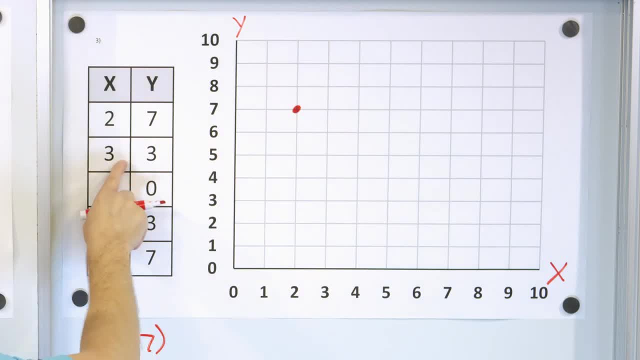 means there has to be a dot right here. Next point: Three: comma three means x is three and y is also three. That means there has to be a dot right there. Next point: Five: comma zero: x is five, which is here, and y is zero. 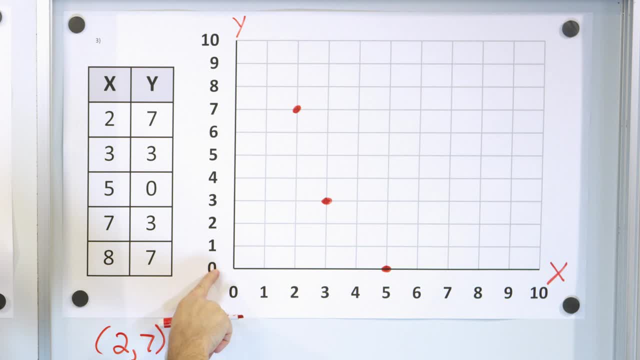 That means there's actually a point way down here. y here is zero way over here. so when I go to x is five, y is zero, it doesn't go up at all because y is zero down here. Seven comma three. You could represent that as seven comma three. 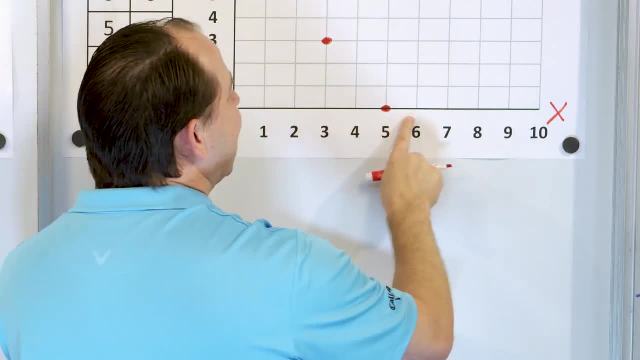 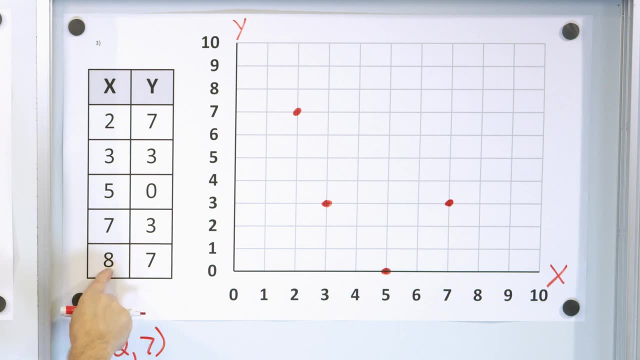 in a parenthesis: x is seven, y is three, x is seven, y is one, two, three means there's gotta be a point like this: Eight comma seven, x is eight, x is eight is way over here and y is seven. 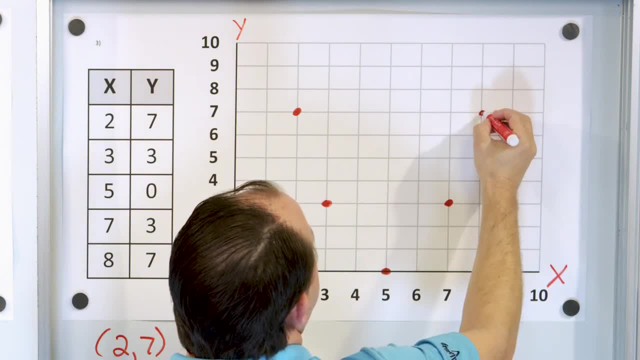 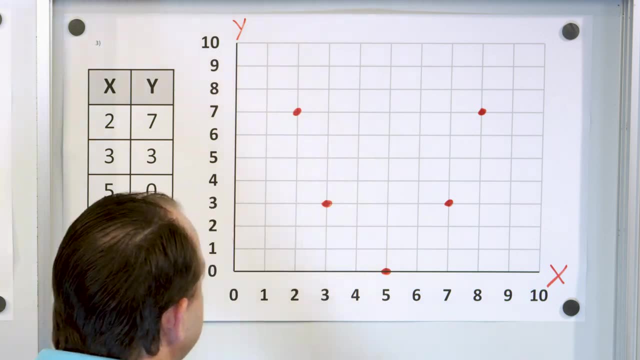 One, two, three, four, five, six, seven means there has to be something here. Now this one's really interesting, right, because this doesn't form a line. I mean, you can try all you want, but it doesn't form a line through all these points. 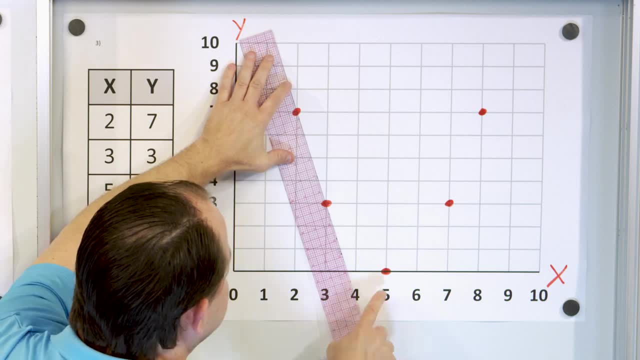 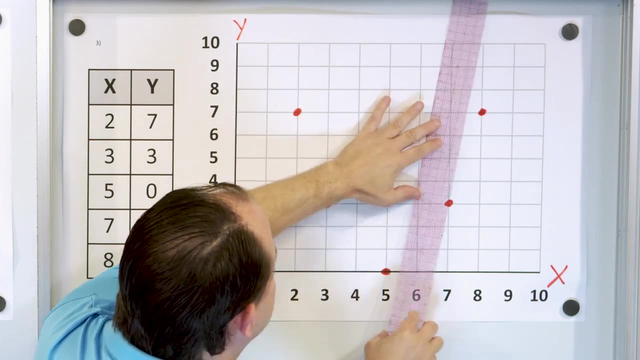 In fact it does. if I go through these two points like this, it doesn't even hit this one. If I go through these two points like this, it still doesn't hit this one. There's no way to even catch these three points. 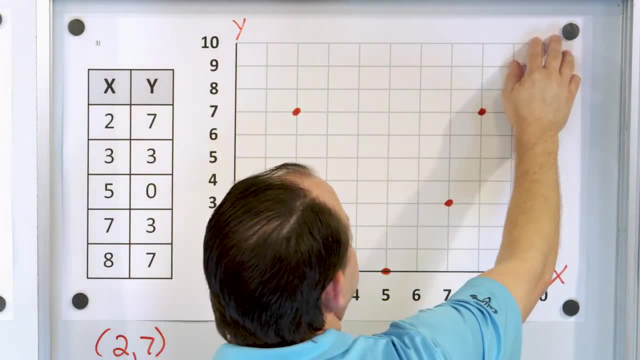 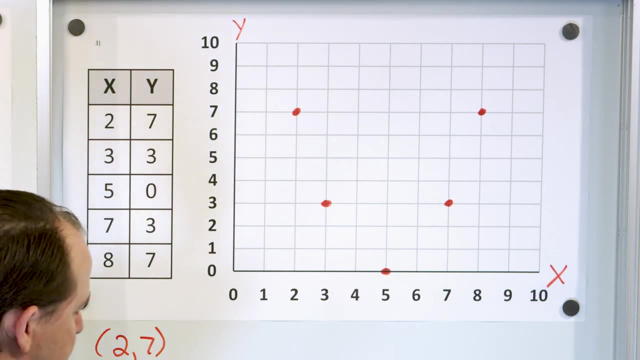 along a straight line. So this does not form a line. So you might say: what kind of shape is this? Sometimes, when you draw graphs, you just have to draw the best curved line that you can through it. Now, this is not gonna be exact. 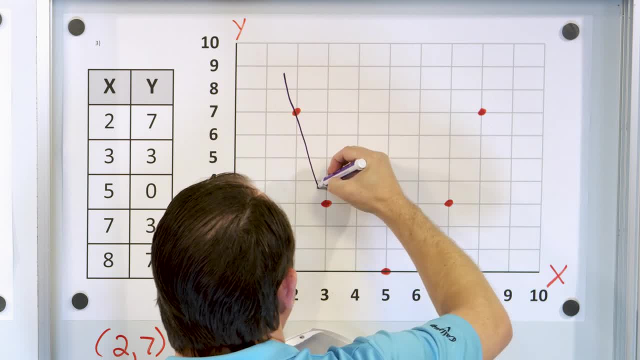 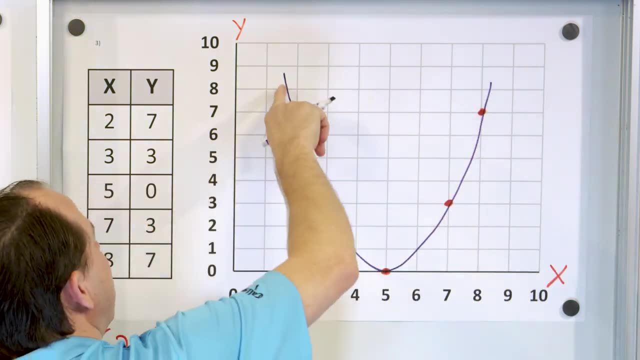 but this line might be something like this: It might go through here, might go through here, hook and curve down and then go up, something like this: Now, of course I went up past the points there. You could put little arrows, kind of pretending. 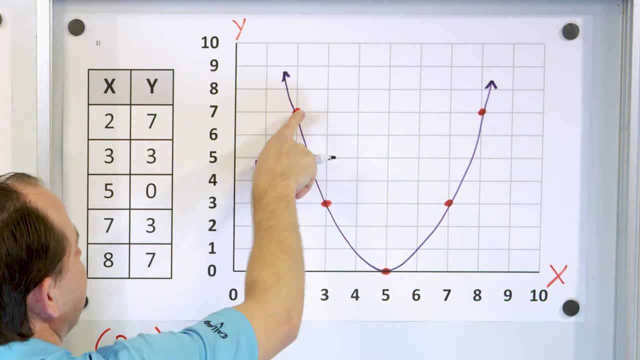 that the graph goes up beyond these points that I've plotted, But really I guess with the data I have, it stops at these points there. Now, this is an interesting shape that we run into all the time in math. You'll see as you learn more and more. 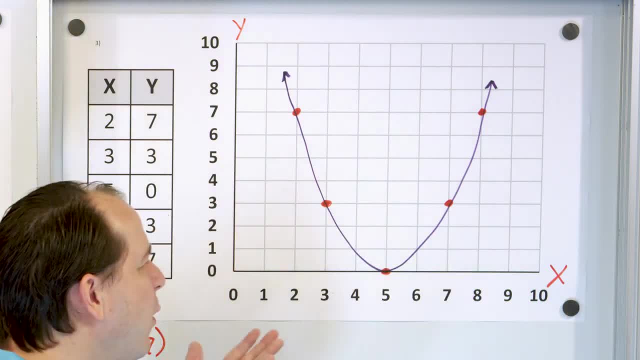 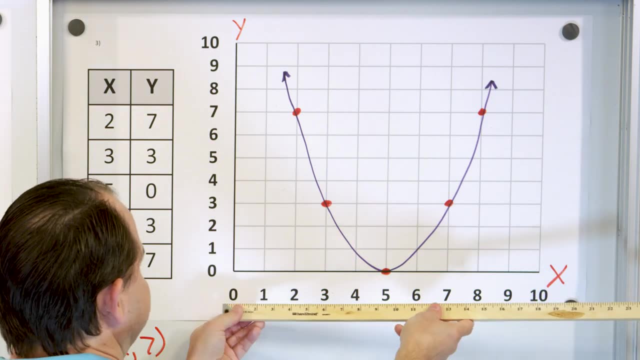 you'll learn about these shapes more and more as we go along. but what could it represent? Okay, what could it represent? Let's go back to our rod example. Let's say that the X direction is telling me how far from the end of the rod I am. 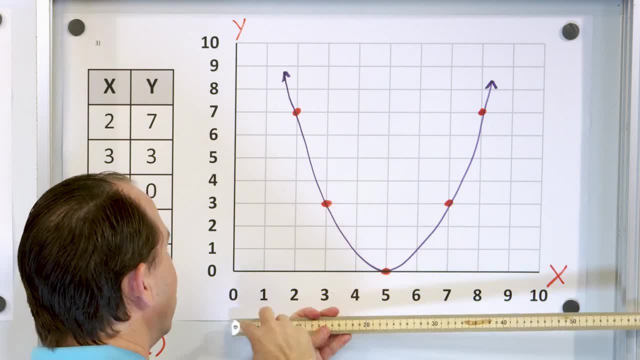 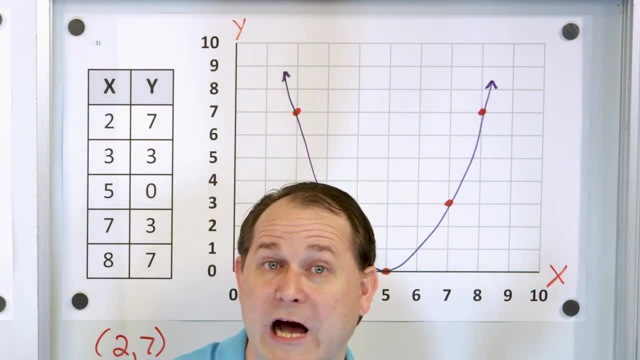 So here's one centimeter, two centimeters, three centimeters, four, five, six, all the way to 10 centimeters right. And then this direction here is telling me the temperature of the rod, right. So let's say that over here, near the end of the rod, 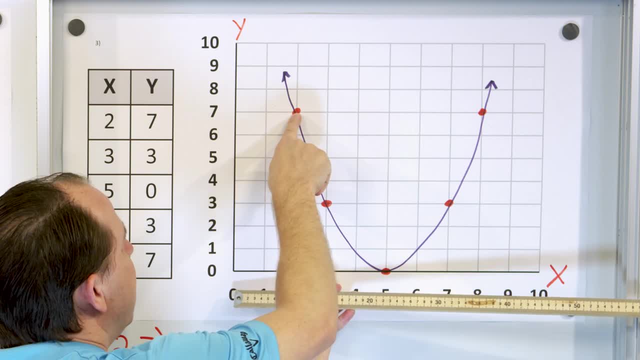 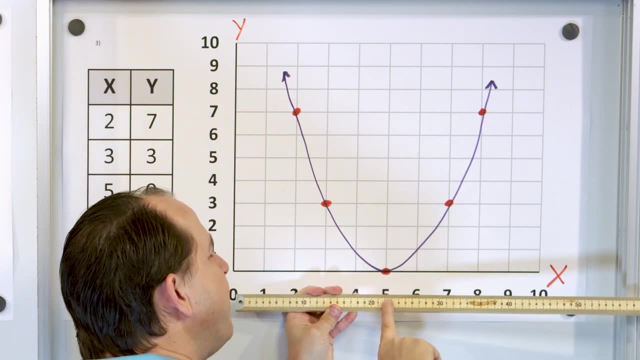 at two centimeters is really high temperature- seven degrees. But then as I go to the right, the temperature is dropping. Then the temperature drops to, let's say, zero And then, as I go past this point, when I get here at seven centimeters, 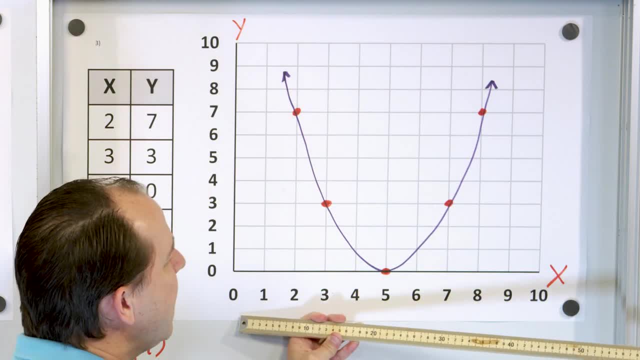 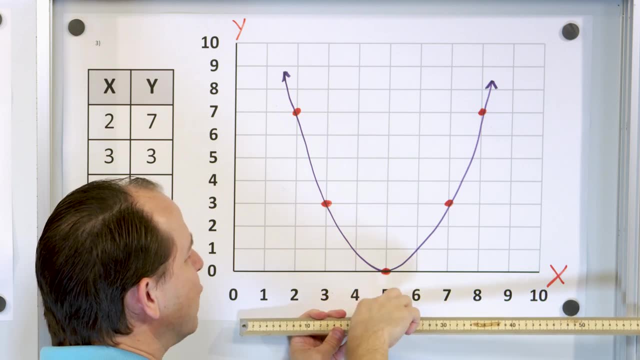 temperature goes up again and then the temperature goes up again. How could that be? I mean, just an example of that. would be what if I had an ice cube? if I put an ice cube right on the center of the rod? 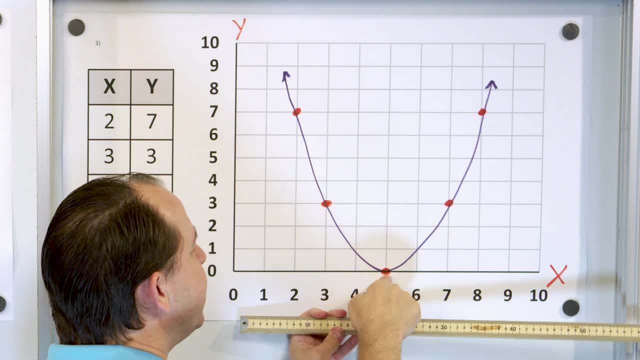 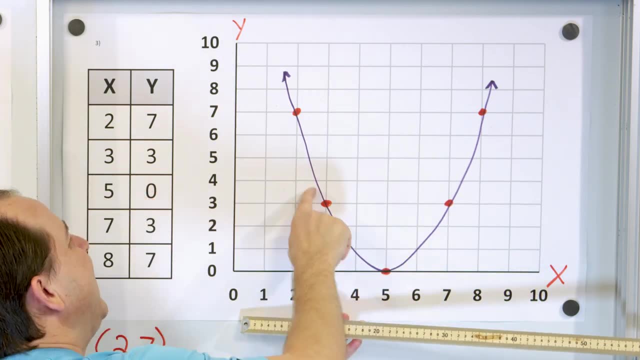 right here. Well, that would mean it's cold right in the middle, so the temperature is low. But as I go just to the left and to the right of the ice cube it's a little bit warmer, And then as I get farther away it's even warmer. 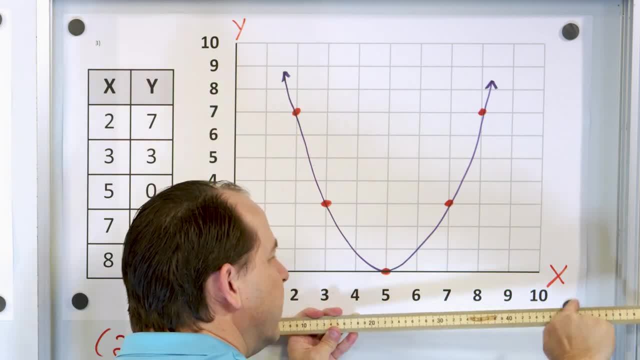 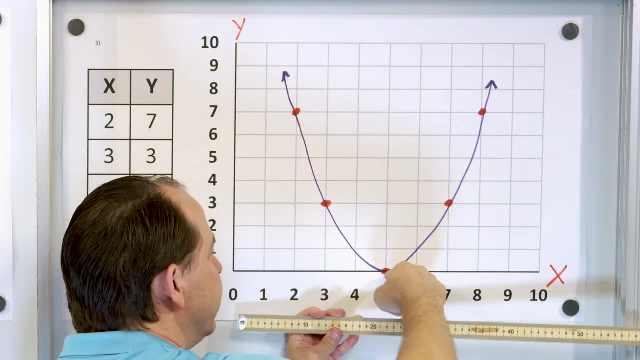 Down here, So this could represent in distance this direction, and then this Y direction is telling me the temperature, which is going down to an ice cube and then going up again as I go again away from an ice cube. So what I'd like to do is take these down. 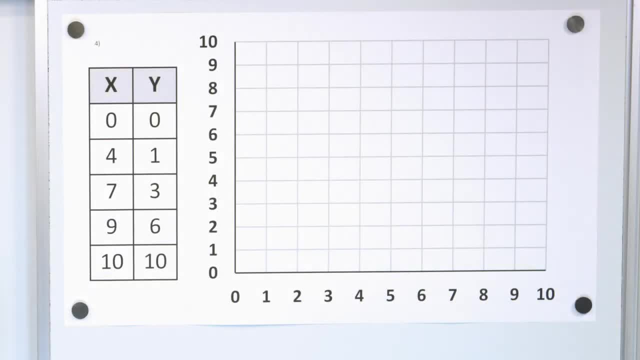 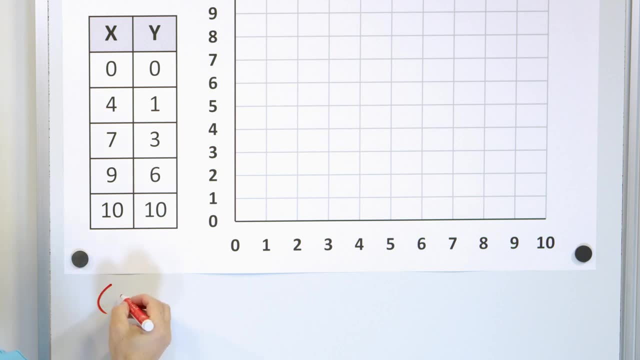 and do three more to give you a little more practice. All right, here's our next problem. This one's also a really cool shape. Let's take a look at the first point. Zero for X and zero for Y, If you wanted to write that in terms of a parentheses form. 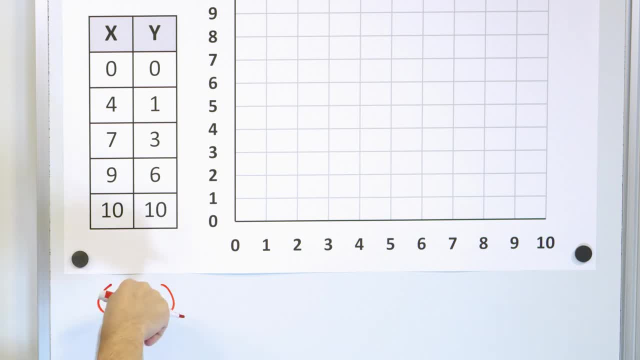 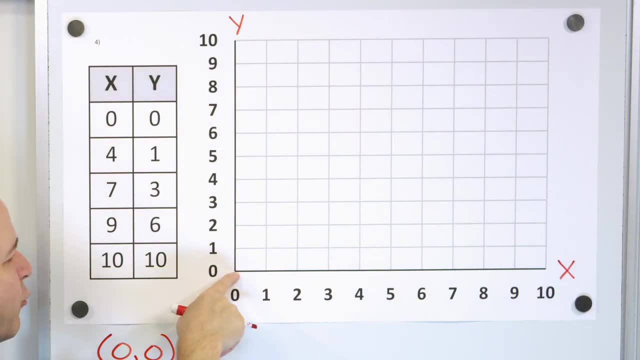 that you see a lot. you'll write it as zero, comma zero. That means X is zero and Y is zero. Well, if the again don't forget, this is the X direction and this is the Y direction. If X is zero, that means I'm right here. 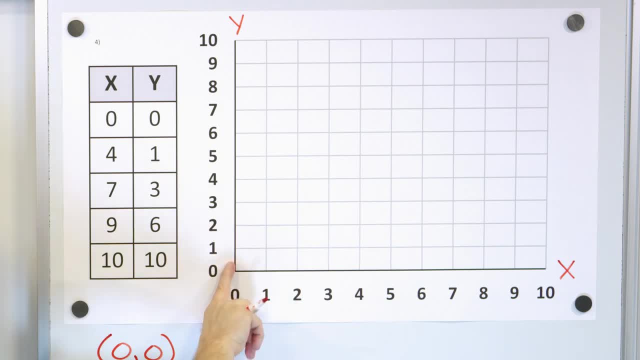 I don't go any direction over here, And if Y is zero, I don't go any direction up. So zero comma zero is right in the corner down here. We call it the origin. Zero comma zero is the origin. It's the lowest or the smallest point. 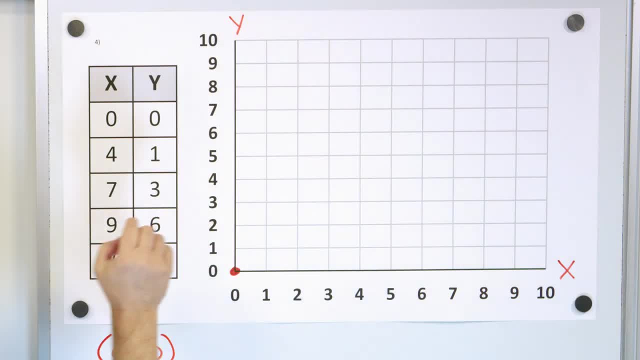 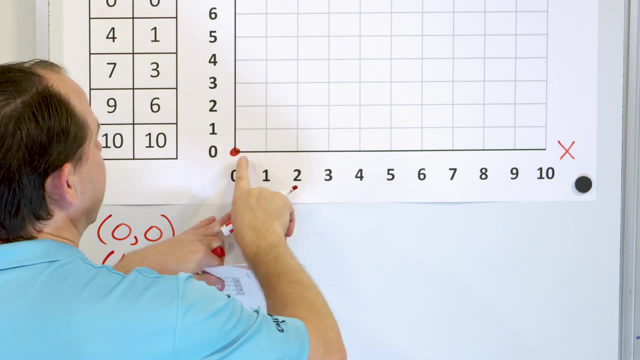 of the coordinate system where X and Y are both zero. All right, So you have a point at the origin. Now you have four comma one. You would write that as four comma one. X is four, Y is one. If X is four, that's four for X, right here? 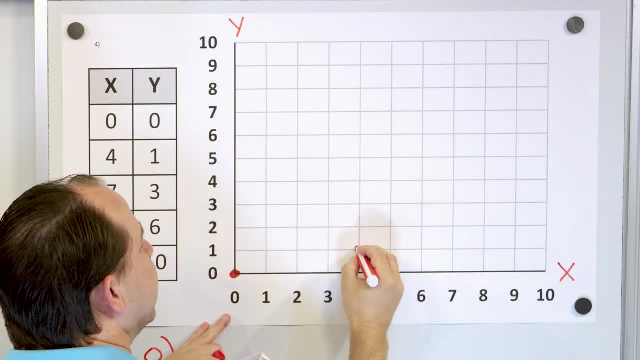 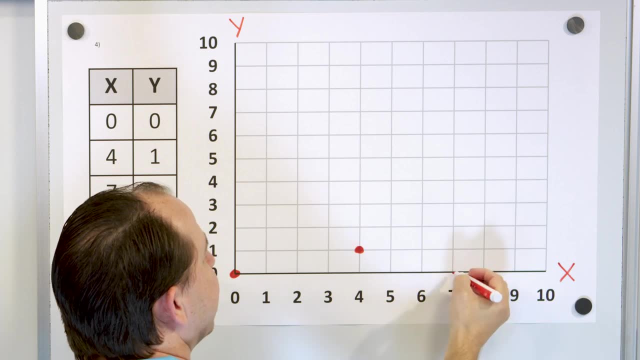 and Y would be one. Y would be going up only one, which would mean there'd be a point right there. Next, seven, comma three. Seven for X and Y, for three. One, two, three Means there's a point right here. 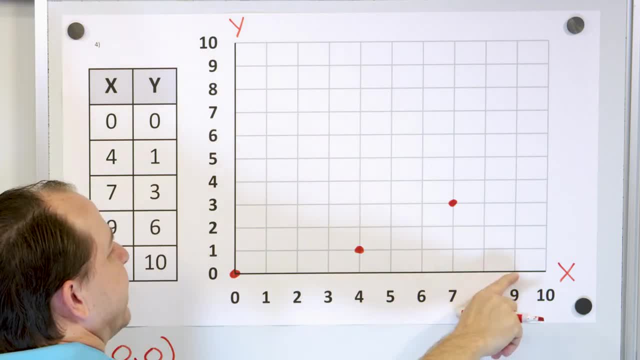 Next nine comma six. Nine for X and six for Y. One, two, three, four, five. six for Y means it would be right here, And then 10 comma 10.. We have 10 over here for X and 10 over here for Y. 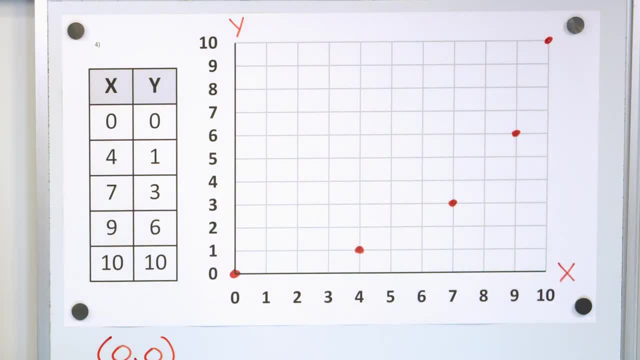 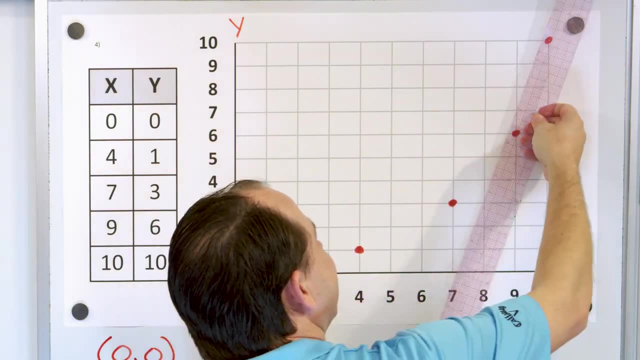 which means there would be a point right here. Now again you have the same kind of problem as the last example. There's really no way to draw a line. I mean you could kind of draw a line this way. You could kind of do something like this: 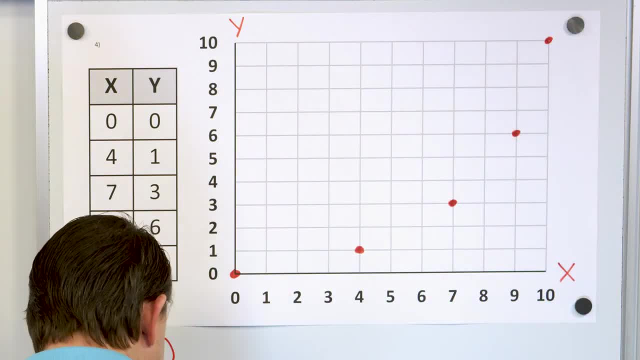 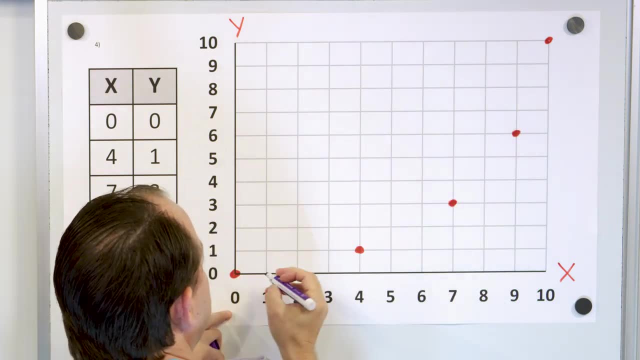 But there's no way to capture all of these points in a line, So it's not a line. Let's draw our best shape that we can through. here Again, Let's try to connect it with a smooth curve, And my curve is not going to be perfect, so please forgive me. 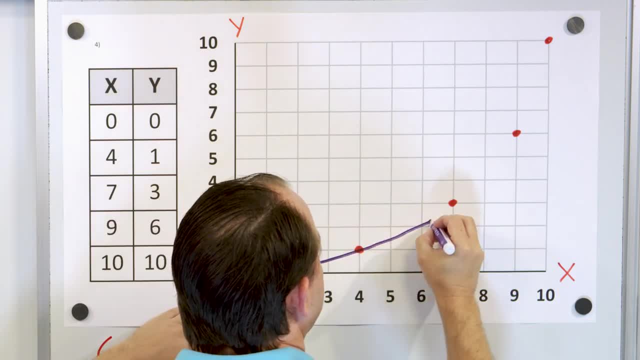 But let's just try to go up. We'll hit this point, We'll hit this point, We'll hit this point And we'll hit this point. That's not too bad. It's a little lumpy, but you get the idea. 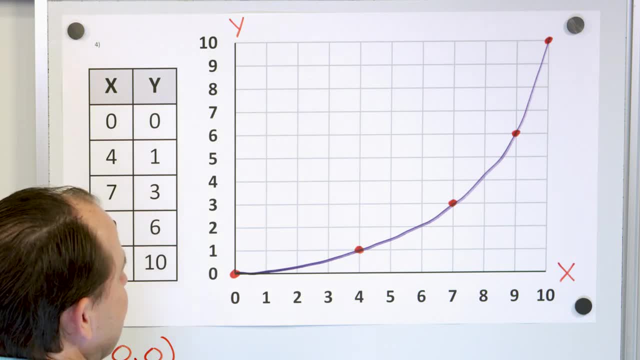 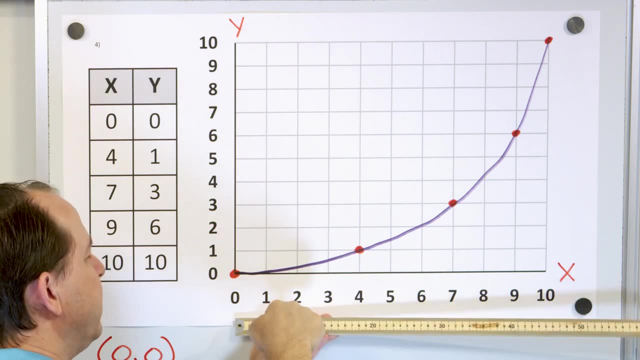 Now what would something or what could something like this represent? Let's say again that we had a rod- And here is the end- at 0 centimeters, And this is 1 centimeter down the rod, 2 centimeters. 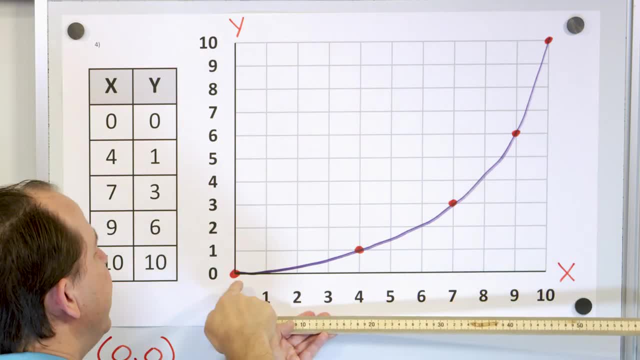 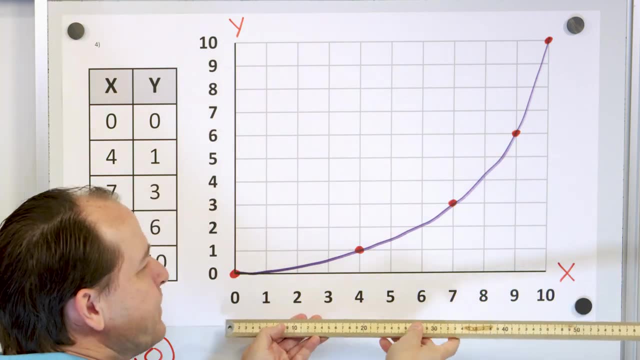 down the rod and so on all the way to 10 centimeters down the rod. This could be the temperature of the end of the rod over here, And this would be the temperature over here at 10 centimeters. Let's say that I had a flame or a blowtorch, just kind of heating. 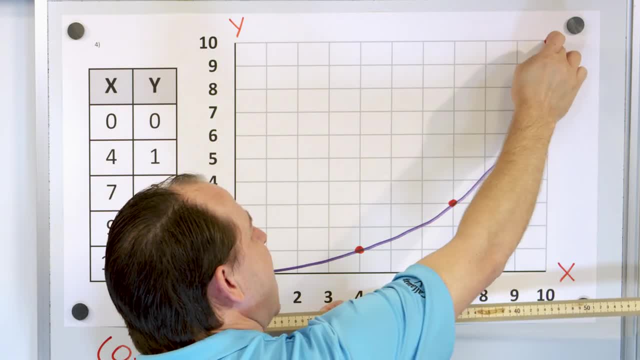 this guy up way at the end, Then the end is going to be really really hot over here at 10 centimeters. really really hot, 10 degrees, let's call it. And then, as I get farther away from the flame, 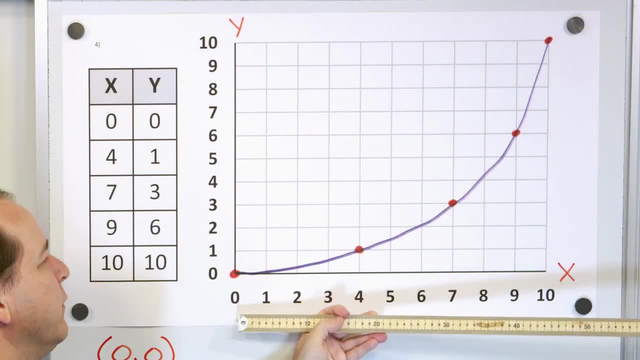 the temperature is going to go down, down, down to, let's say, the end of the rod is at 0 degrees. So this could represent a temperature kind of thing as well. It could represent lots of things. It could be stacking rocks. 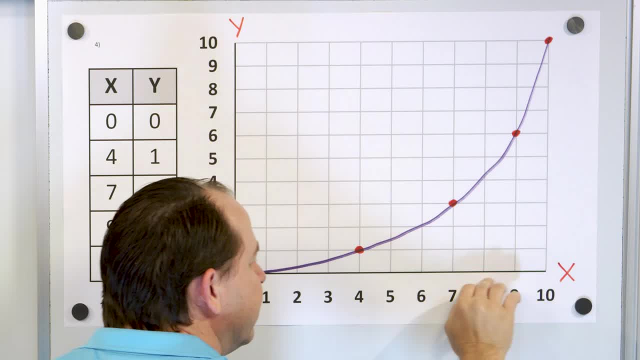 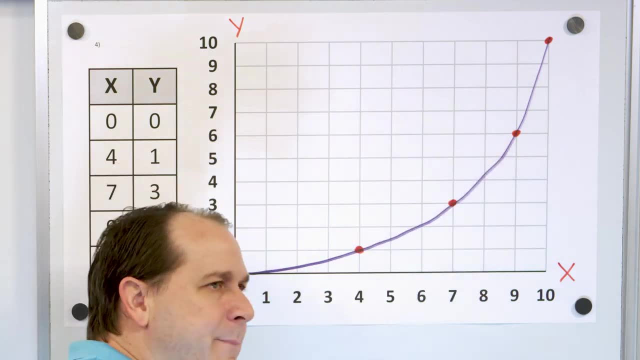 We could also represent it as, let's say, this is time, time in seconds: 1 second, 2 seconds, 3 seconds, 4 seconds, And this is the temperature in the room going up, up, up, up. 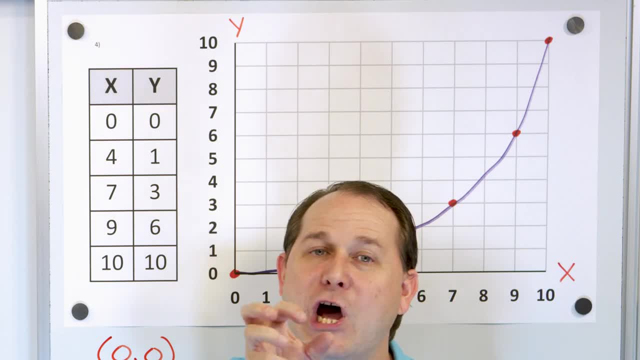 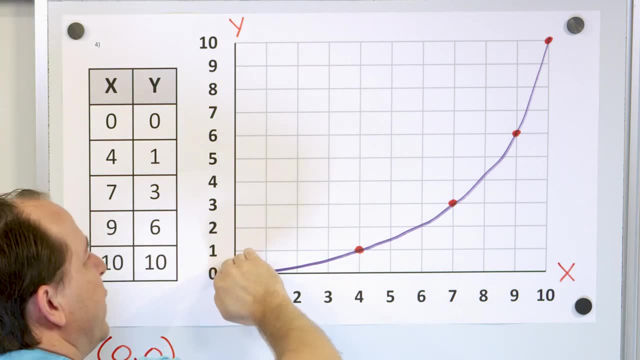 Maybe somebody is turning the knob on the air conditioner, making it hotter and hotter and hotter, But the difference here is notice. in the previous examples, when it was just a line, the temperature would be going up the same amount every second. Here the temperature starts off. really, really. 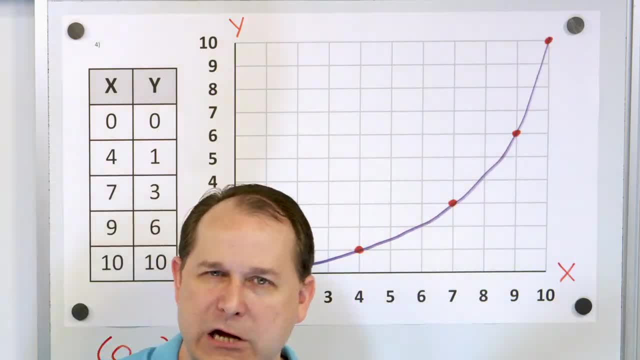 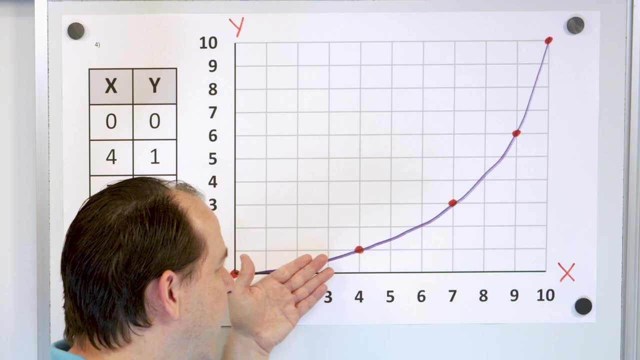 slow and then goes really, really, really fast. So this one obviously is not a line. And if it were temperature, it's not going up the same every second or the same every centimeter or whatever. It's going up much faster at the end here. 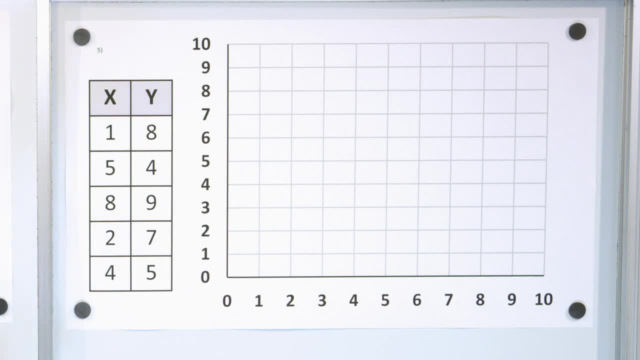 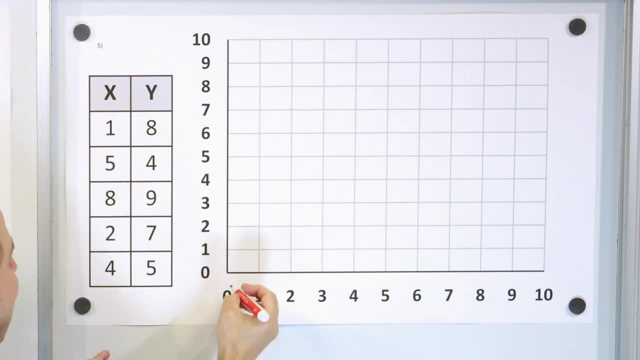 All right, let's take a look at the next one. Let's take a look at this, This one. I'll give you a spoiler. This will be a line, but a different kind of line. Take a look at 1 comma 8.. 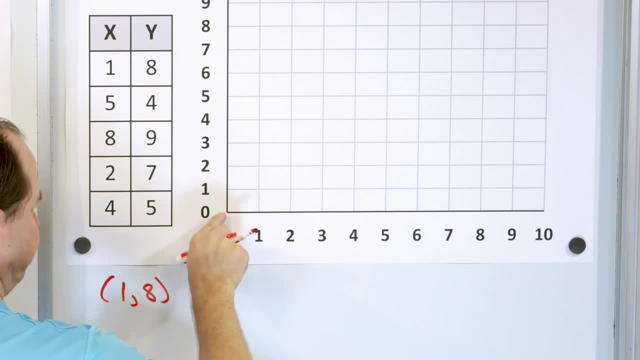 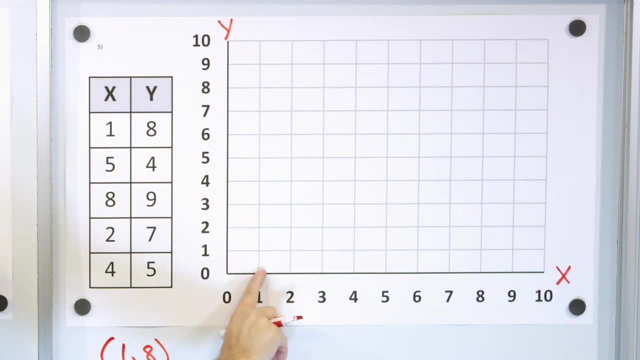 x is equal to 1 and y is equal to 8.. x is equal to 1 is here, Don't forget. This is the x direction, That's the y direction. x is 1 and y is 1,, 2,, 3,, 4,, 5,, 6, 7, 8.. 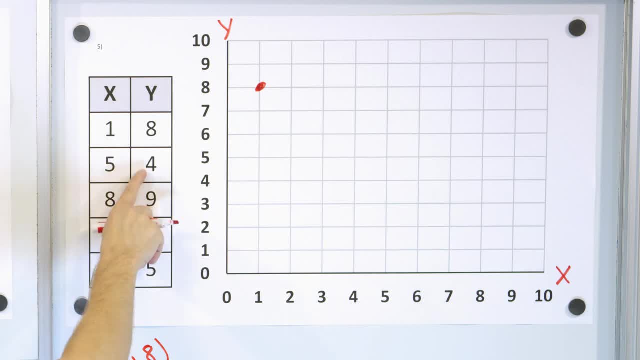 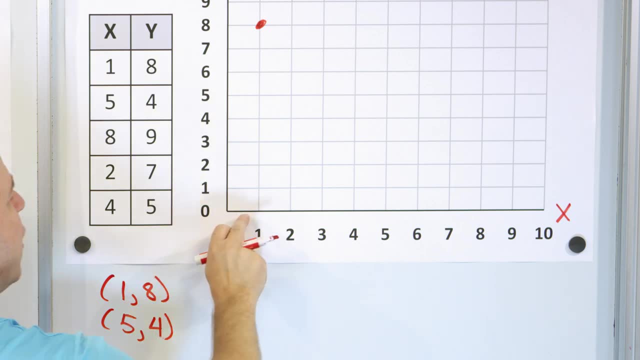 That means there's a point right there. Next, 5 comma 4 is: x is equal to 5 and y is equal to 4.. So 1, 2, 3, 4, 5 for x, 1, 2,, 3, 4 for y. 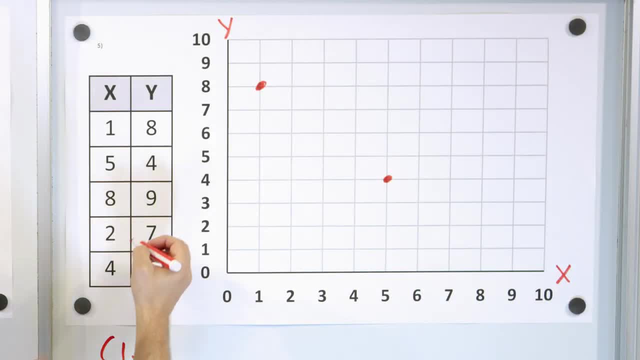 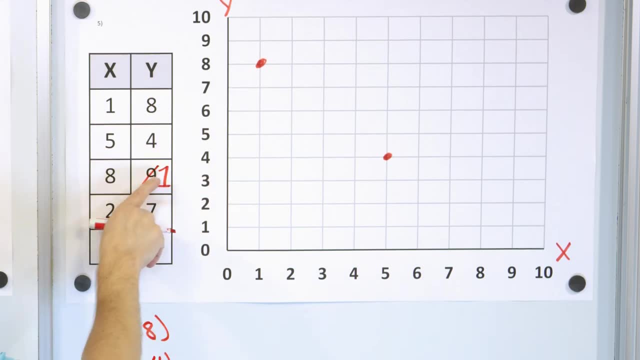 which is a point right here And actually right here. I'm actually seeing a typo here. I'm going to strike through that. That's not the right number. This should be a 1 right there. Sorry about that. So let's plot 8 comma 1.. 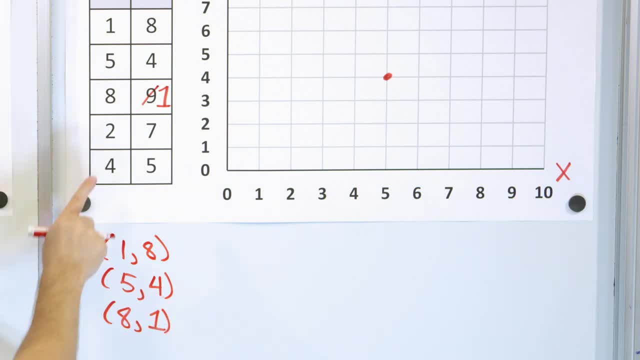 If I were going to write that down, it would be 8 comma 1.. That's the correct point there. So x is equal to 8, which we go over here- And y is equal to 1.. Forget about the 9.. 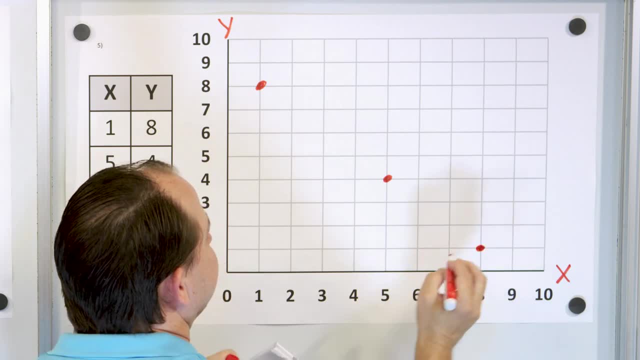 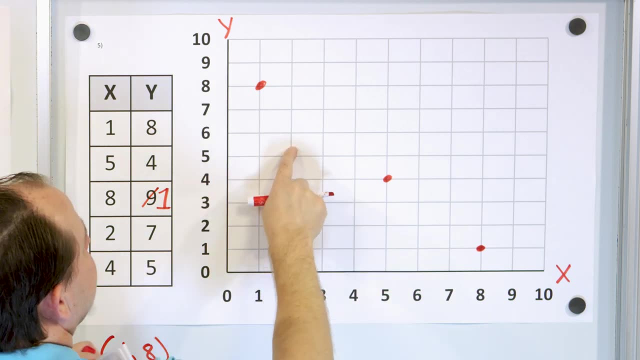 y is equal to 1,, which means 8 comma 1 is a point that lives right there. Next, 2 comma 7.. x is equal to 2.. And y is equal to 1,, 2,, 3,, 4,, 5,, 6,, 7, which. 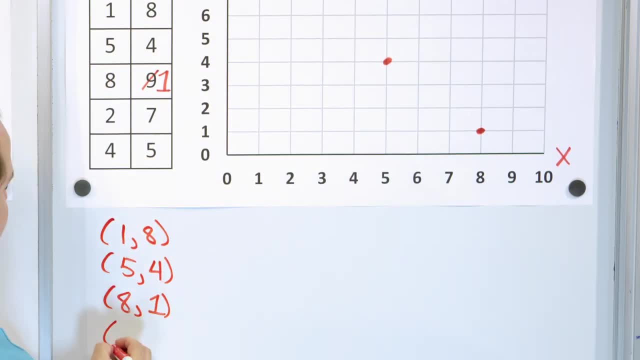 means there's a point right there. And then 4 comma 5.. You can write that as 4 for x, 4 comma 5.. 4 for x, 5 for y, 4 units over for x up, 5.. 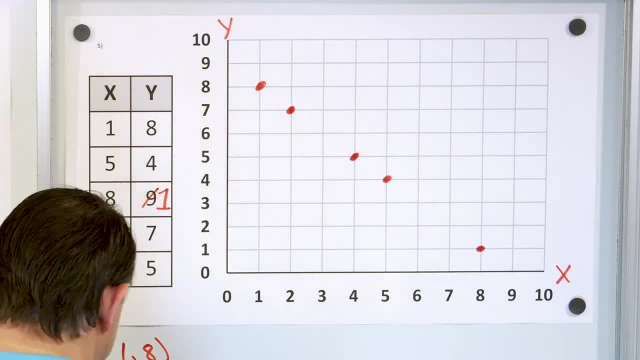 1,, 2,, 3,, 4,. 5 means there's a point right here. Now, this one actually does form a line, And so we're going to connect the dots on that and talk about it a little bit. 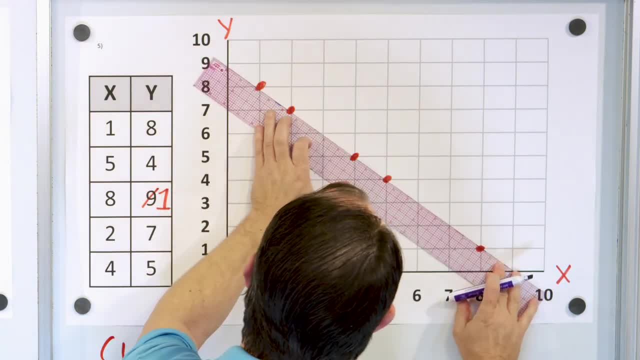 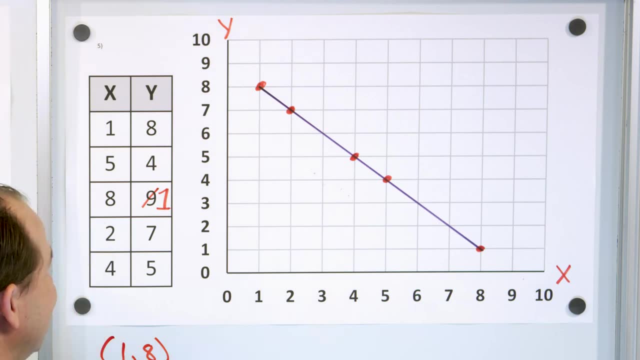 But this line's a little different. It slants the other direction. So let's try to do our best. We'll just connect through here so you can see that that forms an exact straight line. Now the difference between this line and the other lines that we did before. 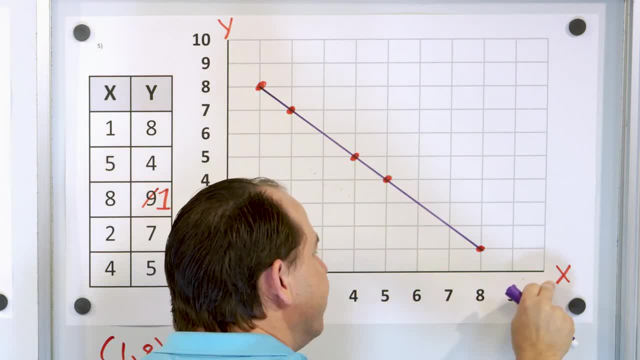 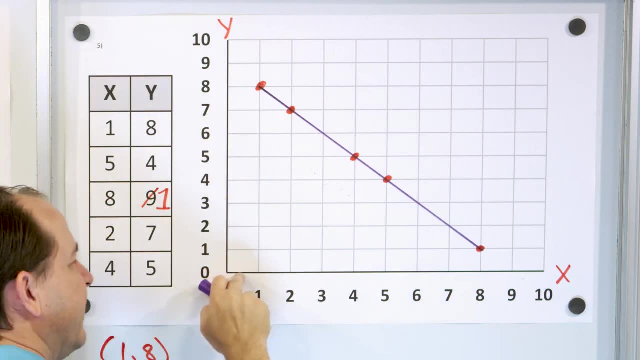 the other lines went this way. So if you think of this being time along this direction and this being temperature- in the other lines the temperature was going up, up up Here- if you think of this as being time and this is being temperature, then what's happening? 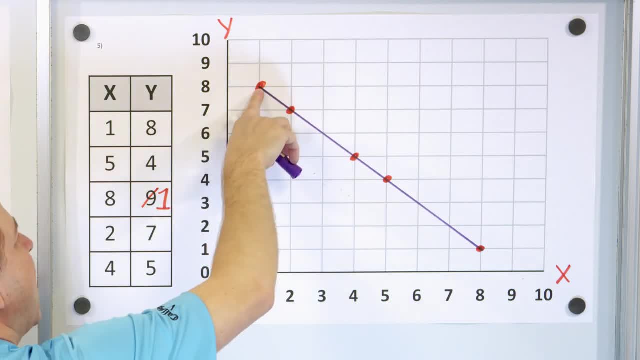 is in the beginning, right when I start my clock. the temperature is high, but it's going down, down, down, down. As the seconds tick by 1 second, 2 seconds, 3 seconds, the temperature is going down, down, down. 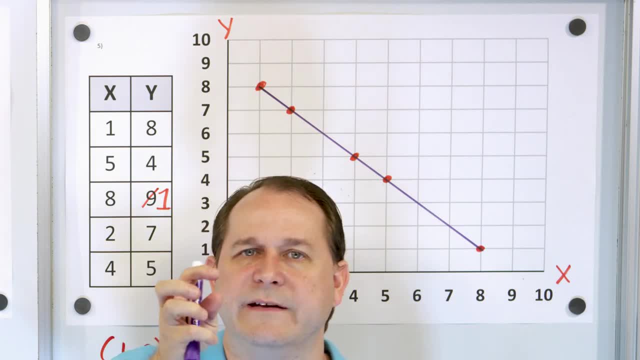 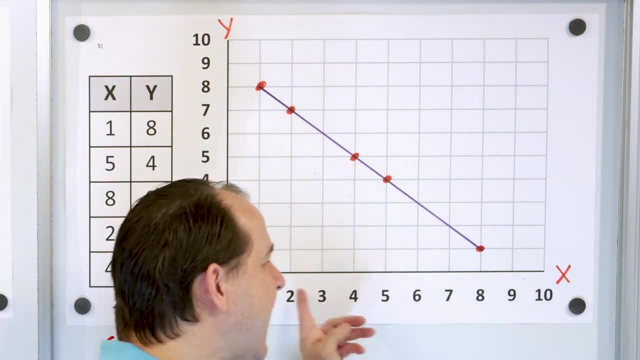 So you can think of this being, you know, like turning the temperature down in a house or something, or putting some kind of cold ice cube on something and watching the temperature go down, down, down as the seconds tick by. Just one example just trying to give you. 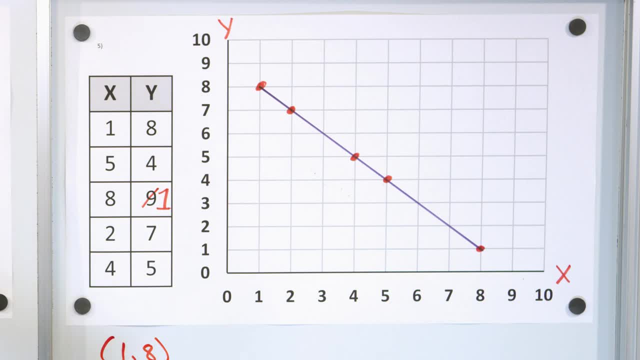 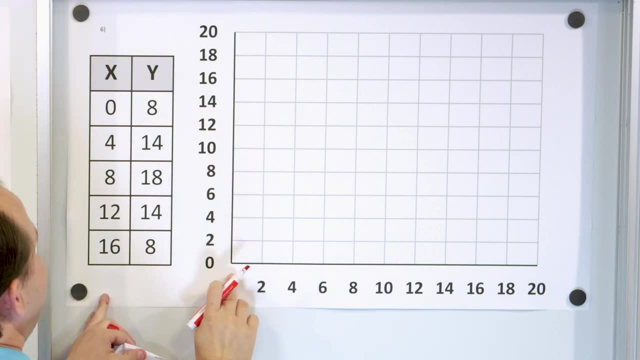 something to anchor this, so you understand what we're using it for. All right, and here is our last one. We have the first point, 0 comma 8.. x is 0, and y is equal to 8.. Now notice, we've changed things a little bit. 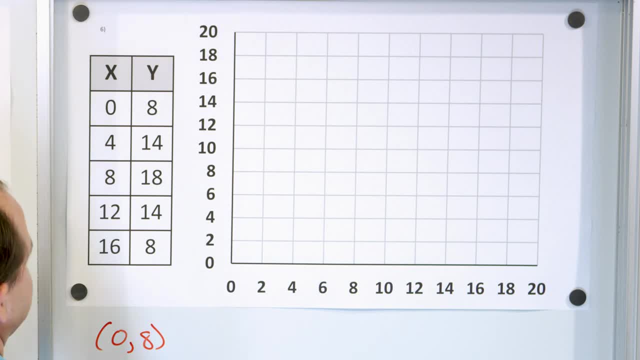 Let's write down 0, comma 8.. In all the previous ones we said it's 1,, 2,, 3,, all the way to 10, 1,, 2,, 3,, all the way to 10.. 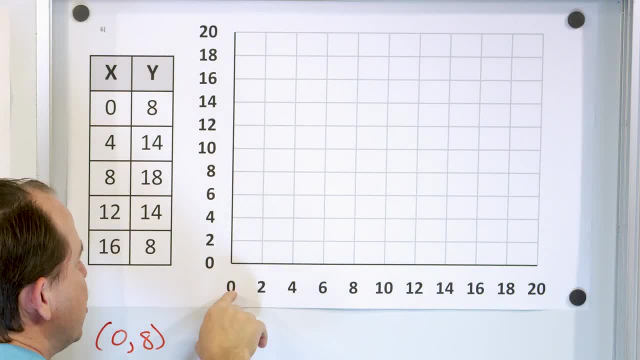 Here we're changing the scale a little bit. Notice it's 0,, 2,, 4,, 6,, 8,, 10, all the way to 20, and same thing up here. Why did we do that? 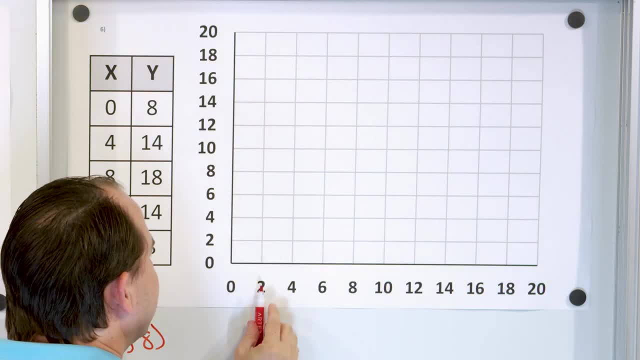 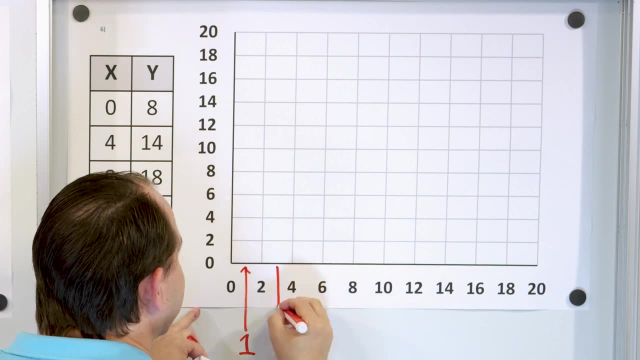 So I could put bigger numbers, But don't forget that right between 0 and 2, like right here, this is the number 1, right. And between 2 and 4, don't forget, right here is the number 3.. 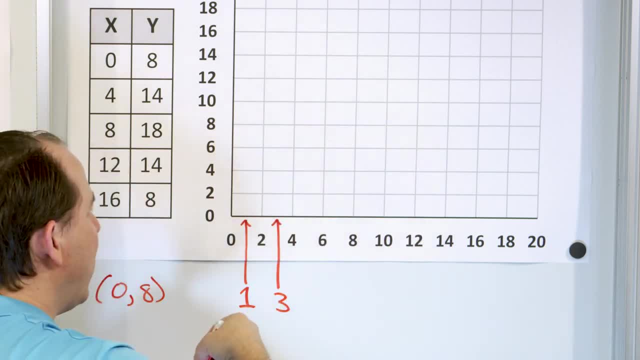 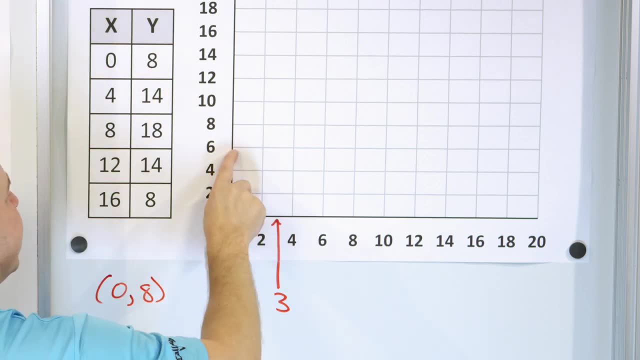 I'm just not writing. I'm writing every number, because then it'll be cluttered. So the way you plot this is: you look at the numbers 0 comma 8, x is 0, right here, y is 8,, 2,, 4, 6, 8.. 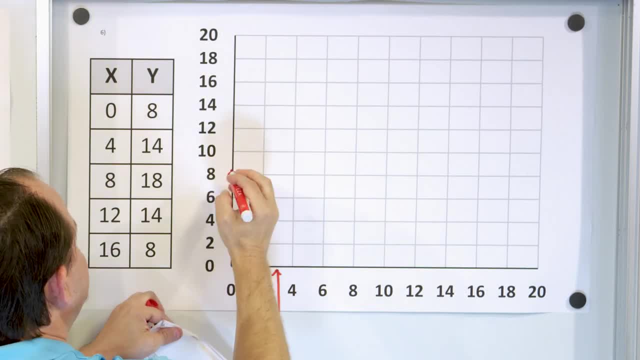 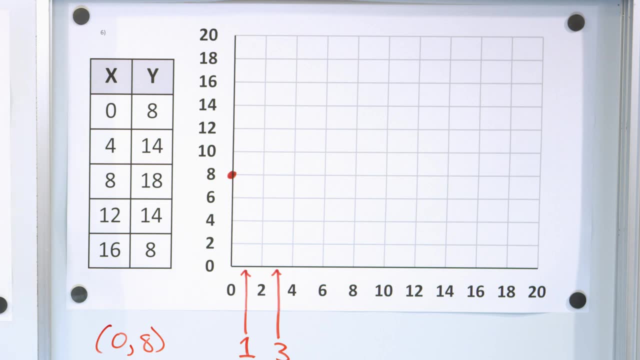 8's right here, And so I just put a dot right there. If you were plotting the point 7,, 0 comma 7, it would be between 6 and 8. It would be right there, But we don't have that here. 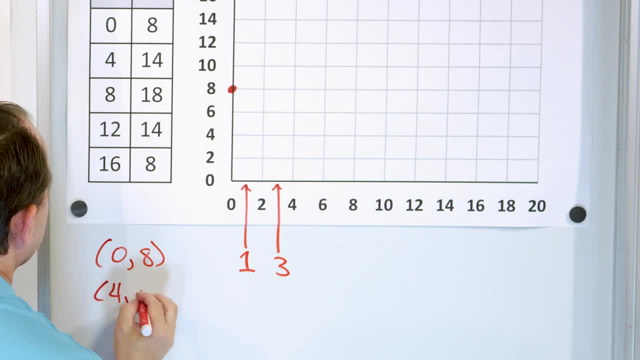 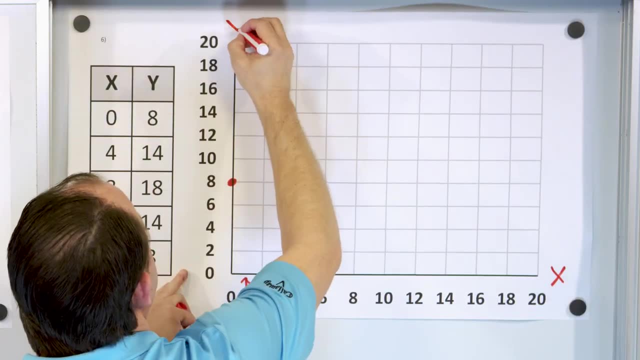 4 comma 14, that means x is equal to 4, y is equal to 14.. So x is equal to 4 is right here. Don't forget: this is the x direction And this is always the y direction. 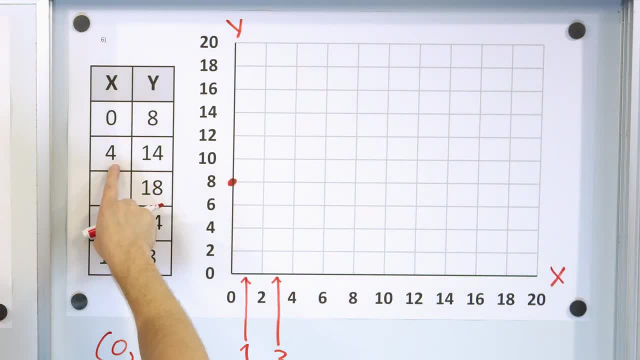 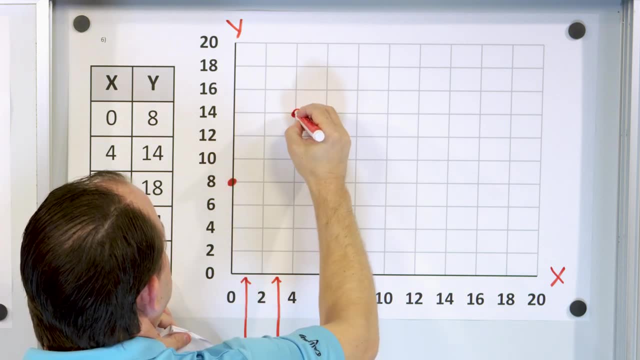 It's always like that when graphing. So we have 4 comma 14.. Here's 4. And we go up until we read 14 off in this direction, which means there is a dot right there. Next we have: x is equal to 8, y is 18.. 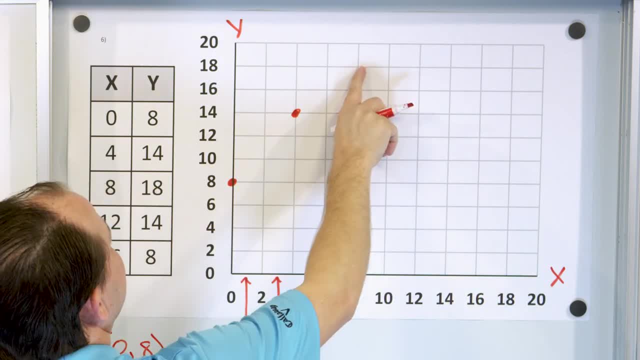 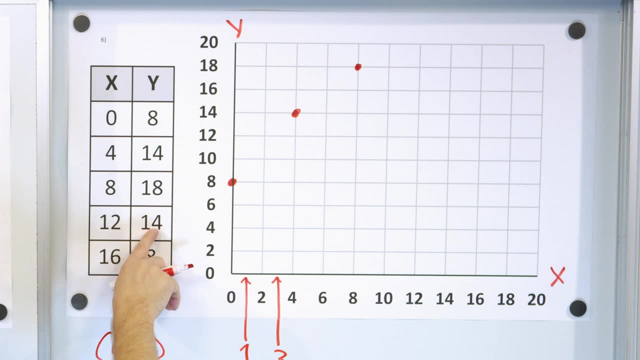 Here's: x is equal to 8,, y is equal to 18.. You just go up until you read 18 there And you put a dot right there. Next We have 12.. 12 comma, 14, 12 for x. 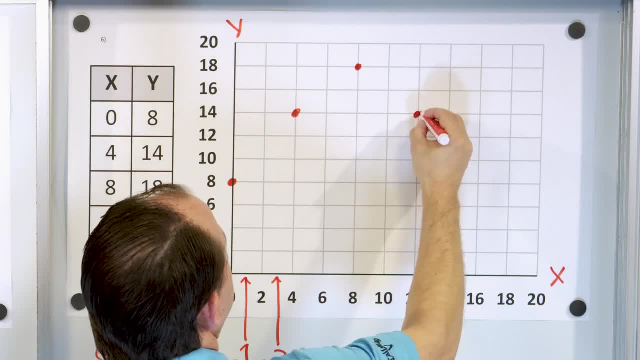 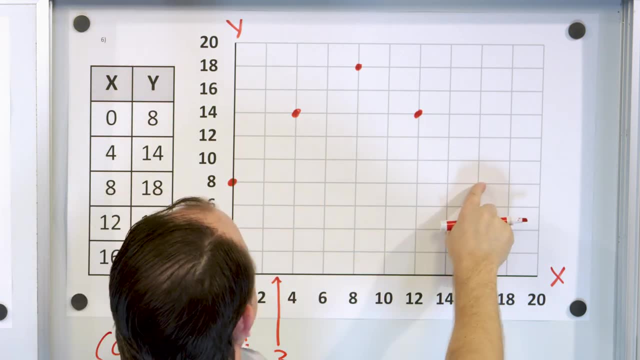 And then we go up for 14, which means we land right there, put a dot right there, And then 16 comma 8,, 16 for x go to 16.. And then 2,, 4,, 6,, 8 means I have a dot right here. 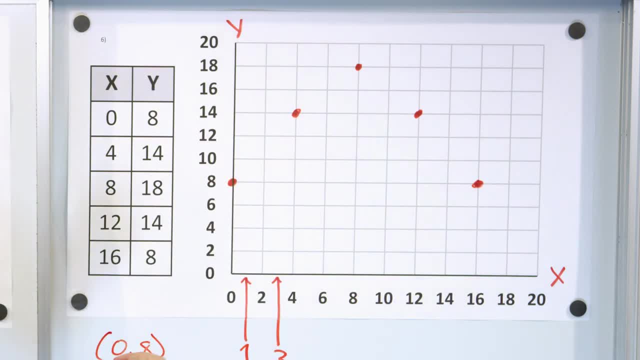 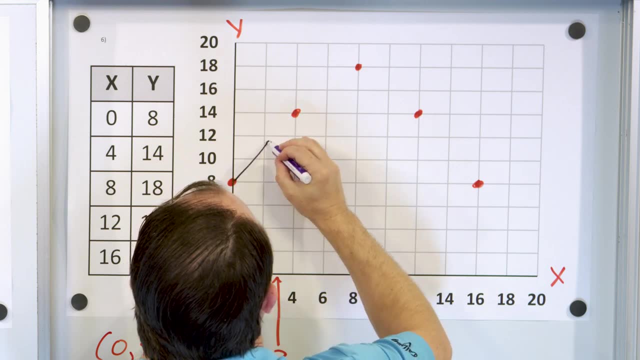 So again, these are not going to obviously form a line of any kind. You can't draw a line there, And I'm not going to draw a perfect curve either, So what you do is just try to kind of go through there. It's a curved kind of deal. 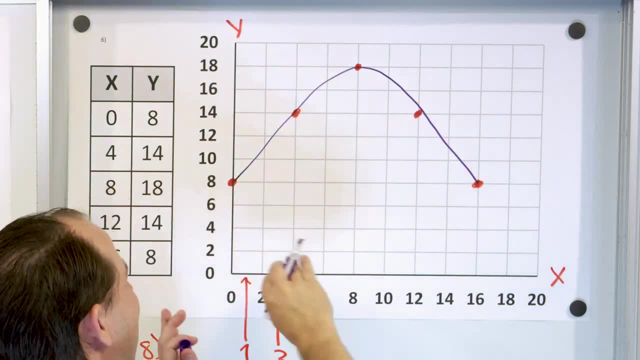 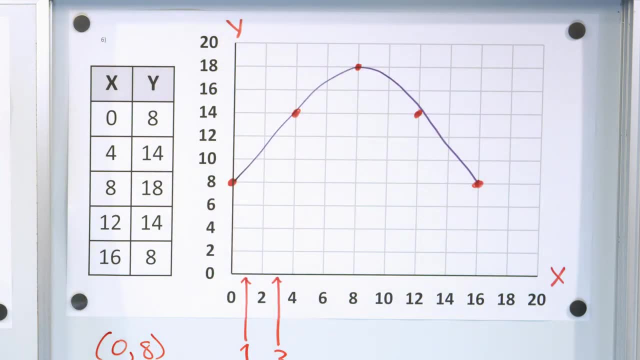 And again, I didn't go through all the points exactly, But you could see it kind of goes upside down. It's not going to form a straight triangle, It's going to do some kind of curved thing over here. And what could this represent? 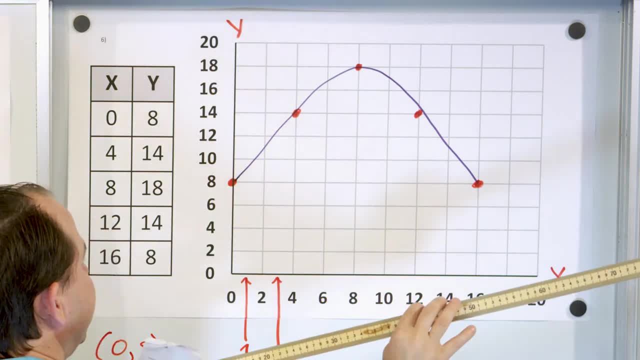 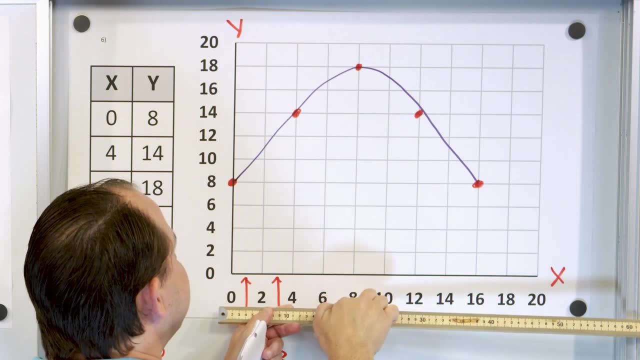 Just off the top of my head. let's say, you have a rod here, right a rod, And you have a blowtorch right in the middle, right here, making it really, really, really hot. So at this distance, 8 centimeters in, 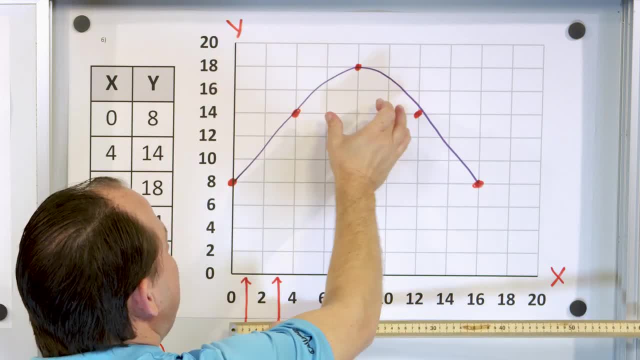 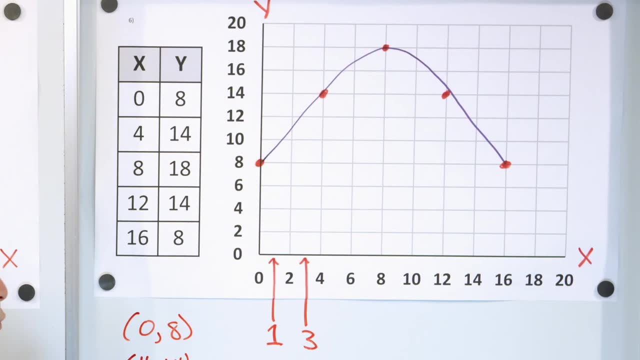 it's really, really hot if this is temperature, And then on either side of the flame it's getting colder And colder. That's why it's going down. So what we use graphs for, the reason why we plot points and we connect the dots, is because when we see pictures,